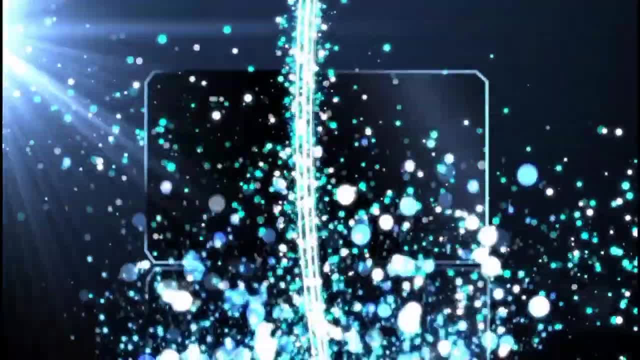 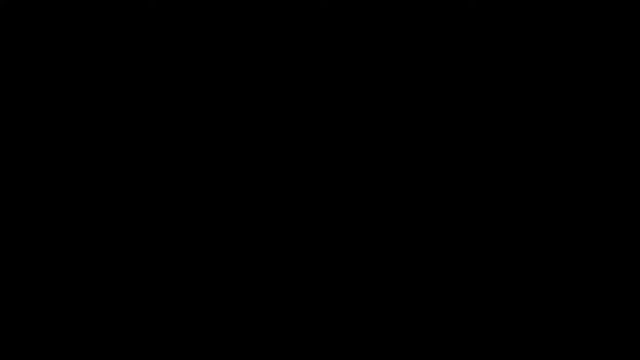 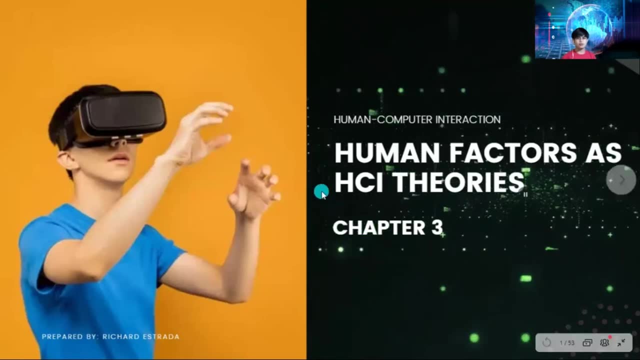 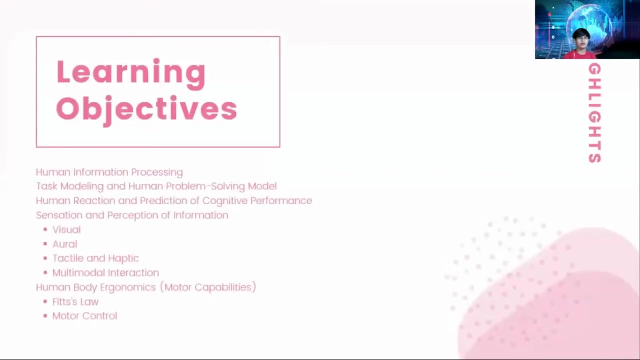 Hello everyone and welcome again to human computer interaction. and we are now in our chapter three and for this chapter we will be learning the human factors as HCI theories. Okay, so our learning objectives are the following: human information processing- we're going to discuss that one task- modeling and human problem-solving model. human reaction: 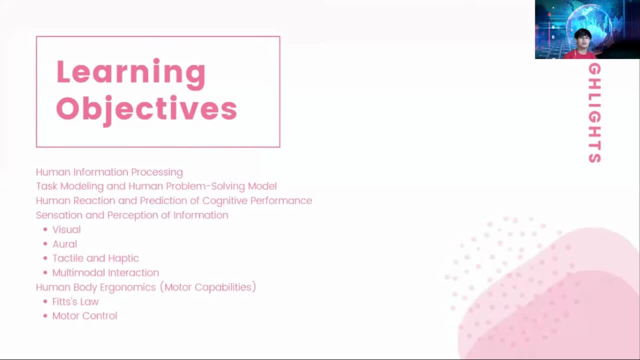 and prediction of cognitive performance, and also sensation and perception of information. that includes the visual, oral, tactile and haptic multimodal interaction, and also we're going to discuss the human body, ergonomics or the motor capabilities. that, what is the law is all about. and then the motor control. Okay, so I hope you're going to learn something. 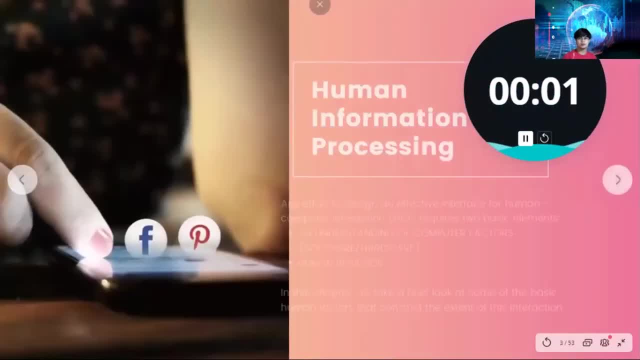 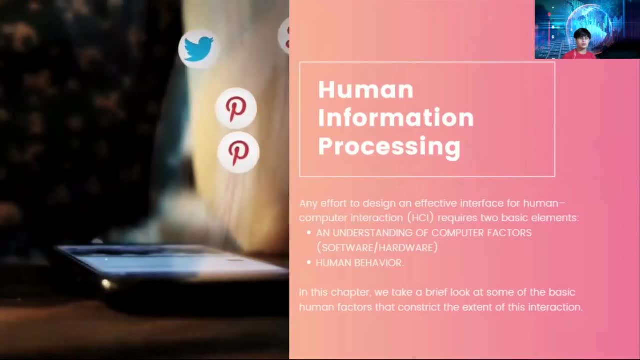 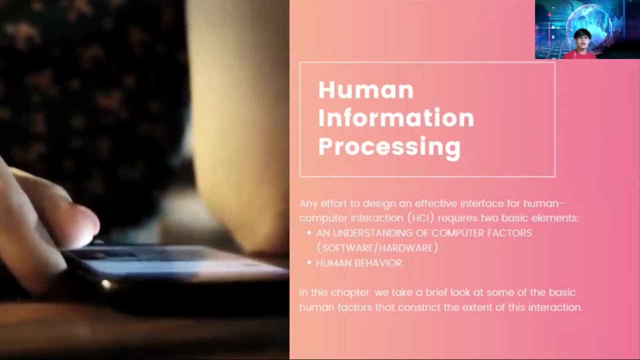 from this video. Oh wait, okay, so the human information processing. so I believe that you are familiar with this, with how the information will be influenced by a human being. Okay, so any effort to design an effective interface for human-computer interaction, or HCI, requires 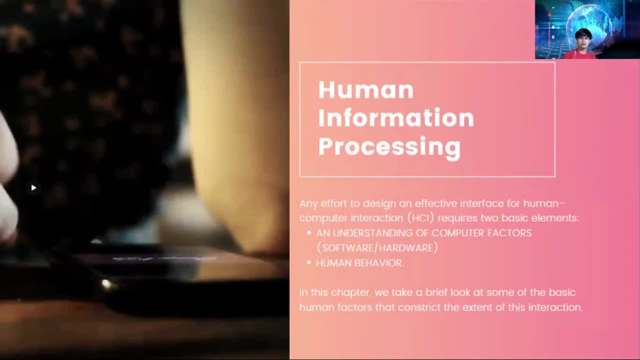 two basic elements. Okay, you need to understand the computer factors: the software and the hardware. Okay, so you should have a little bit idea on how computer works. Okay, what is the software? What is on hardware? What are the different parts of the computer? Okay, and then? 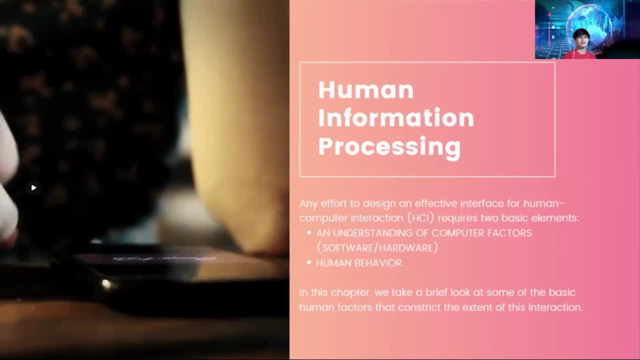 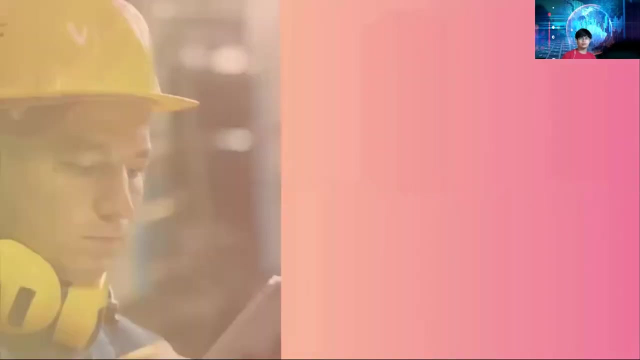 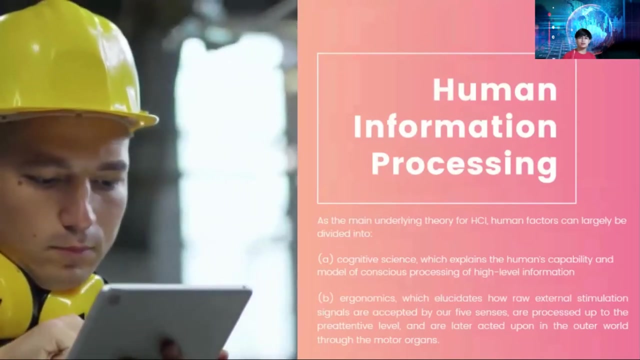 of course. next is the human behavior, your behavior, the user's behavior. Okay, so in this video we're going to look at the some basic human factors that can constrict the extent of this interaction. Okay, so, as the main underlying theory of HCI, human factors can largely be divided into: 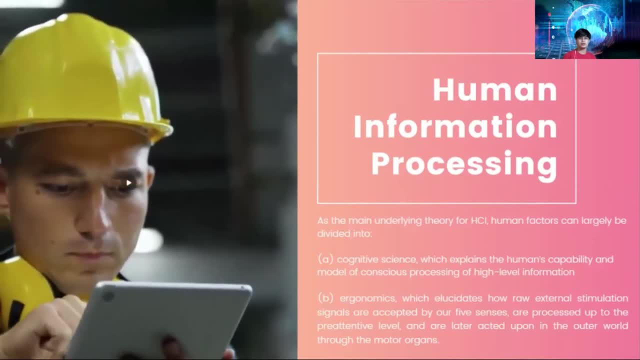 so these are the human factors. First is the cognitive science. Okay, so the cognitive science is a model of conscious processing of high-level information, Okay. when there is a processing of a high-level information, that is called the cognitive science, Okay. and when you say ergonomics: 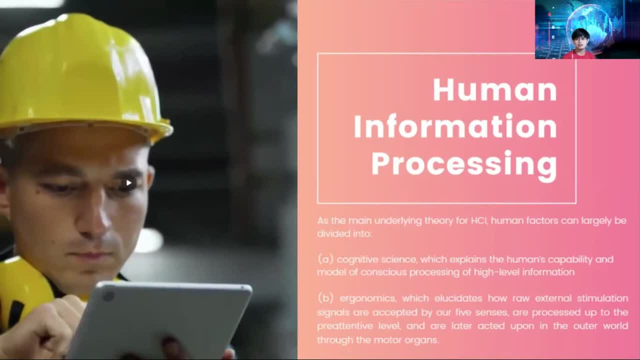 which elucidates how raw external stimulation signals are accepted by our five senses. Okay, so we're going to be discussing the different senses. Okay, on how users, how humans, interact with the computers or any devices. Okay, and that is what we called the ergonomics. Next, 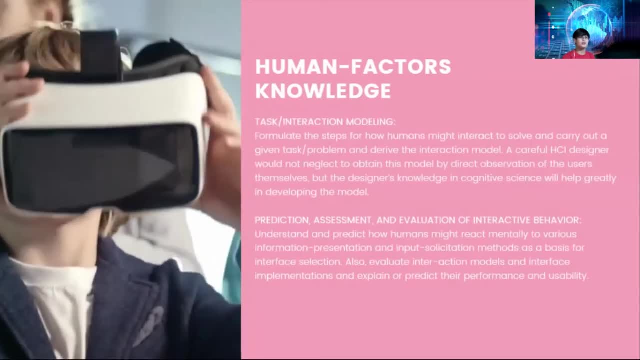 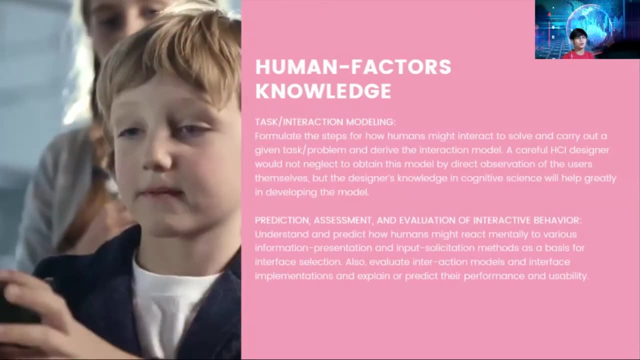 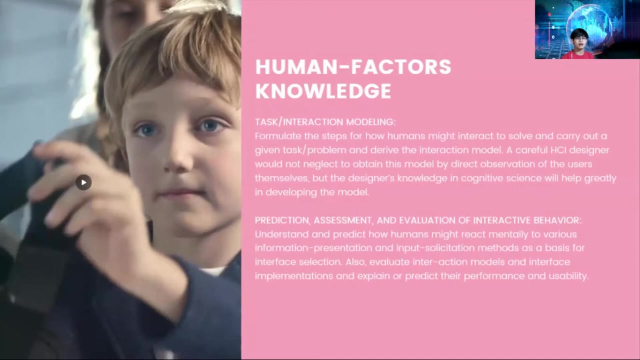 Okay. so we're going to take a look now at the different human factors: knowledge, Okay. so first is the task or interaction. So when you actually decide to design system, you need to, of course, evaluate now what would be how the user is going to interact. So you need to create some. 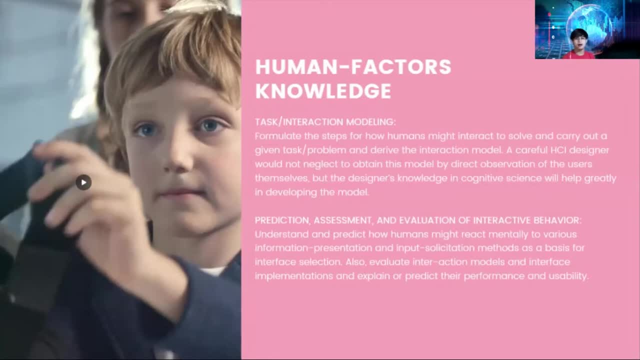 model. Okay, so formulate the steps of how human might interact to solve and carry out a given task or problem and derive the interaction model. Okay, so a careful HCI designer would neglect to obtain this model by direct observation of the users themselves. but the designers knowledge in cognitive science will help greatly in developing. 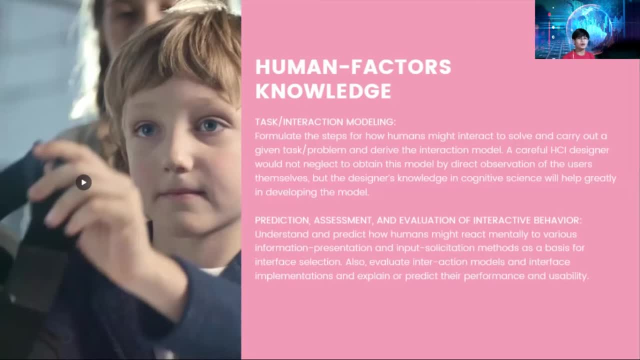 the model. okay, so you need to, of course, again identify what would be the different task or what would be the expected output of the created system. okay, next is the prediction, assessment and evaluation of interactive behavior. okay, so you need to understand and predict how human might react mentally. 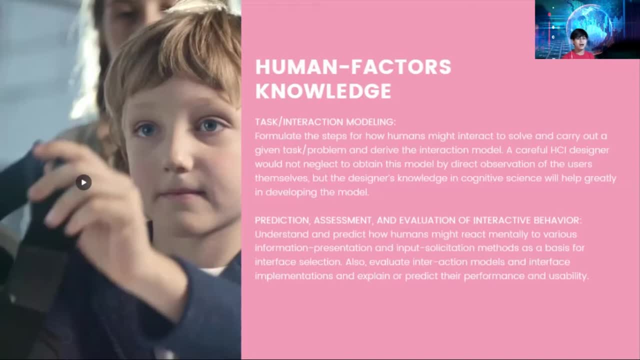 to various information, information presentation and input solicitation methods as a basis for interface selection. okay, and also evaluate interaction models and interface implementations and explain or predict their performance and usability. so you need to know how to predict, you need to know how to assess and evaluate. okay, so that's you know. I believe it's understandable that we need. 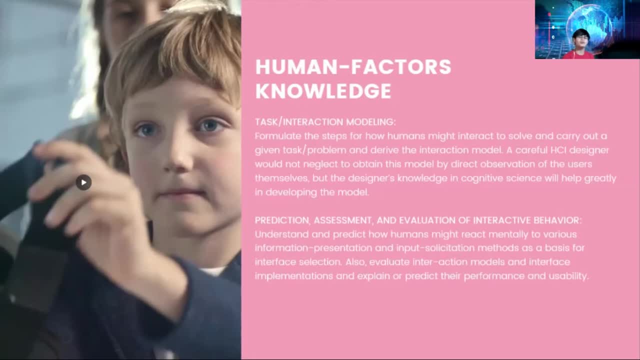 a system you should be thinking about. oh, what if the user will then do this? we're gonna do that. no, what? what would be the positive and negative scenario? okay, so let us say there's a login button. no, the login button will, of course, allow the users to log in. okay, when he click that and once after they click the user. 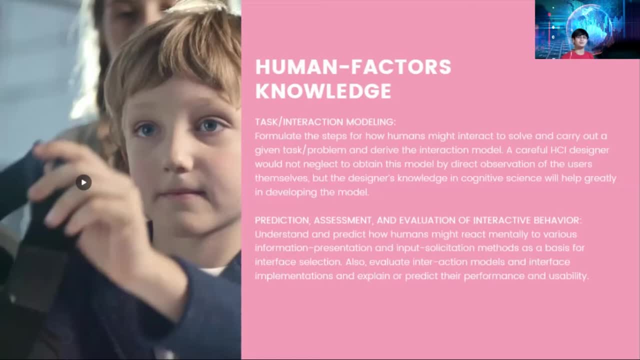 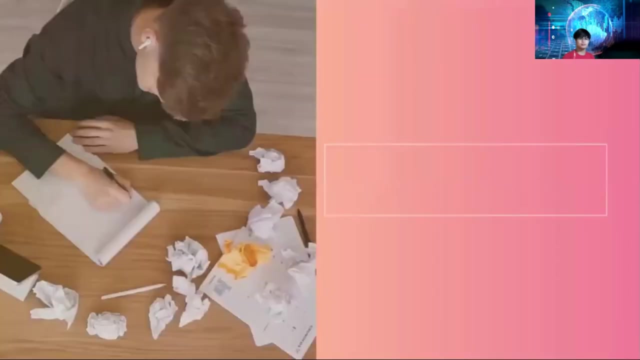 login button, what they say, what is your function? so you need to know, okay, what would be the interactive behavior between the human, the user, and your software or your system. and more on the design, okay. next is the task modeling and human problem-solving model. next is the task modeling and human problem-solving model. 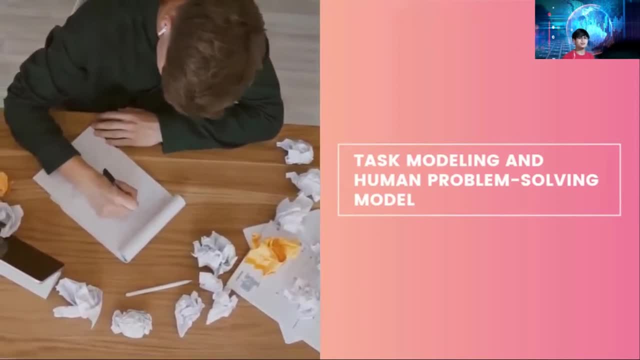 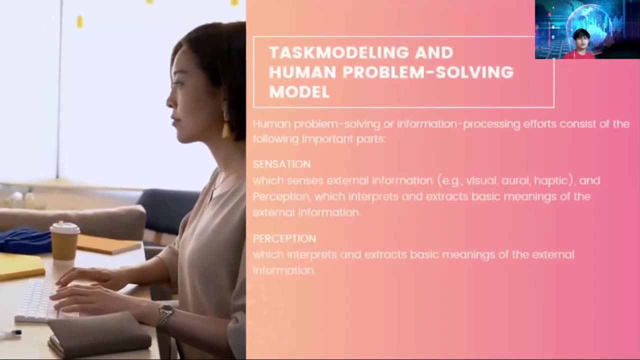 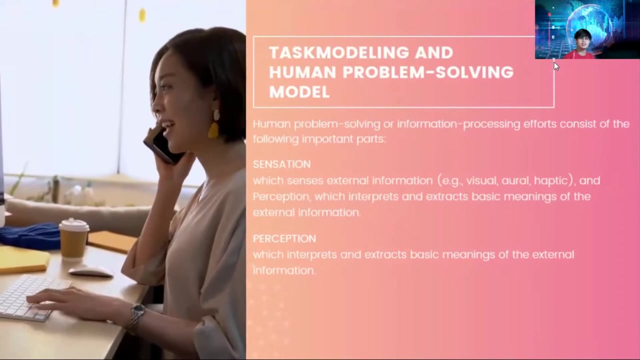 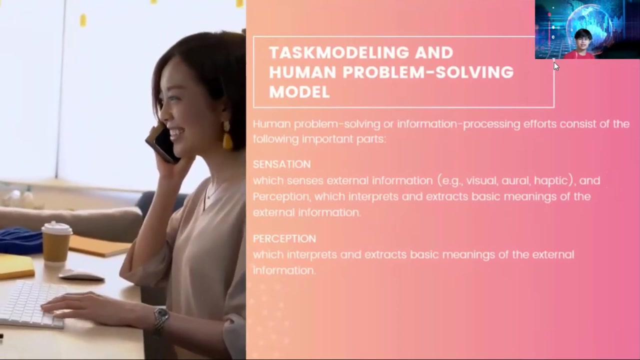 okay, how to model task and very different from human problem-solving model. so human problem-solving or information processing, wait guys, if we're of the following important parts, okay, take note. sensation, which senses external information: okay, example: visual, oral and haptic. and visual, oral and haptic. 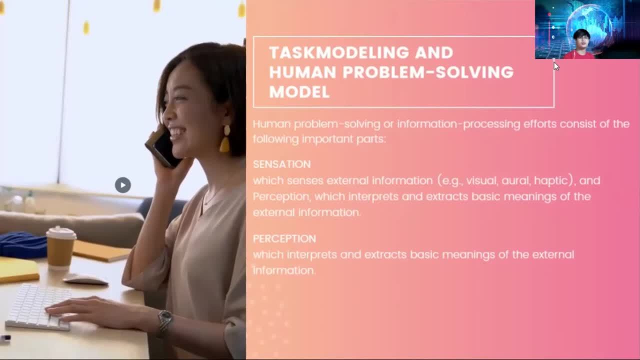 for the sense of, you know, visual, hearing, sound, touch, something like that- and perception. okay, the perception, which, okay so, which interprets and extracts basic meaning of the external information. okay, so, this is difference between the sensation, again, which senses external information, and then the perception is which interprets and extracts the basic meaning. okay, your. 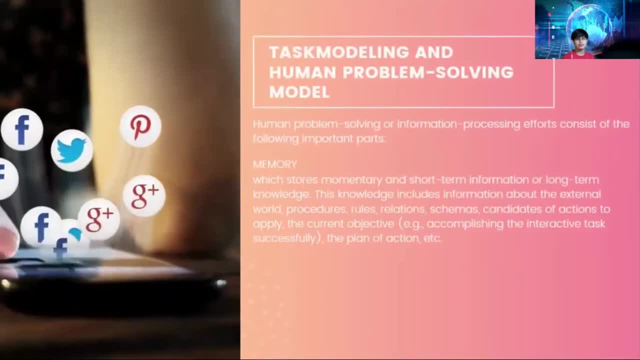 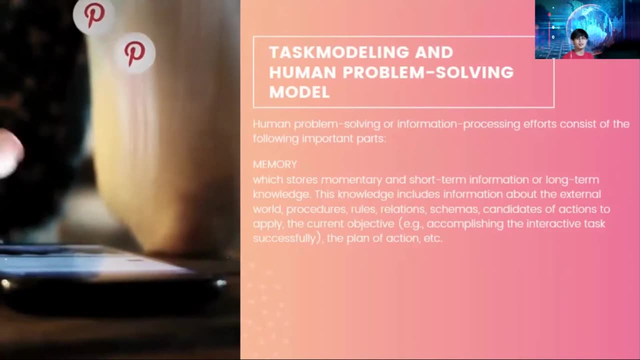 Mhm perception. yes, is this that? and next memory? okay, so, of course, although that's all of us, humans has memories. even computer has memories, which stores momentary and short-term information, or long term knowledge. okay, so this knowledge includes information about the external world, Procedures, Rules, Relations, Schemas, Candidates of actions to apply and Current Objective. 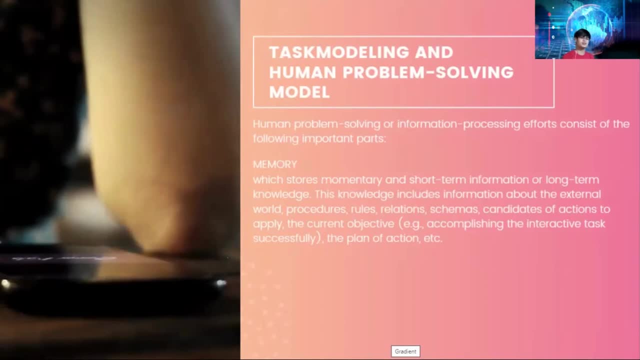 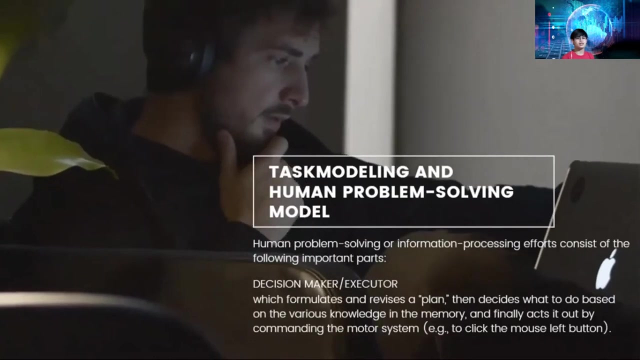 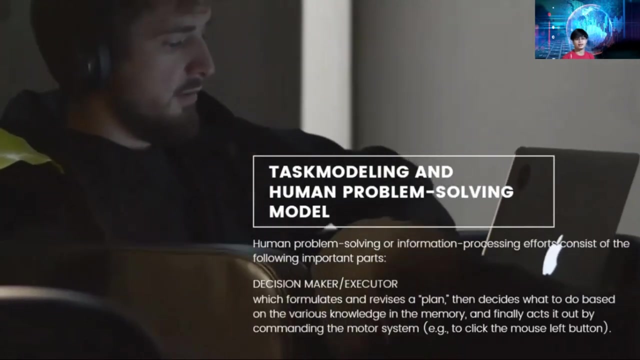 For example, Accomplishing the Interactive Task Successfully, or the Plan or Action or Etc. So that's pretty basic, okay. Next, Decision Maker or Executor: The Decision Maker. this will formulate and revise a plan, then decide what to do based. 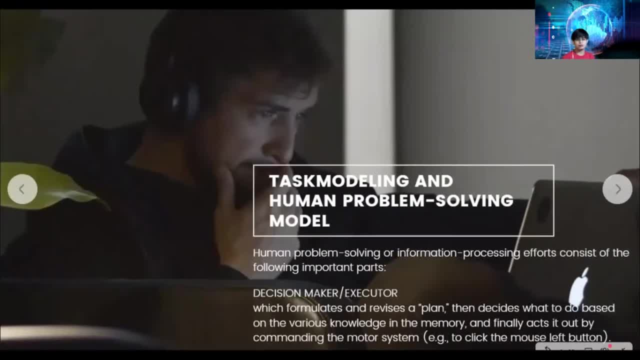 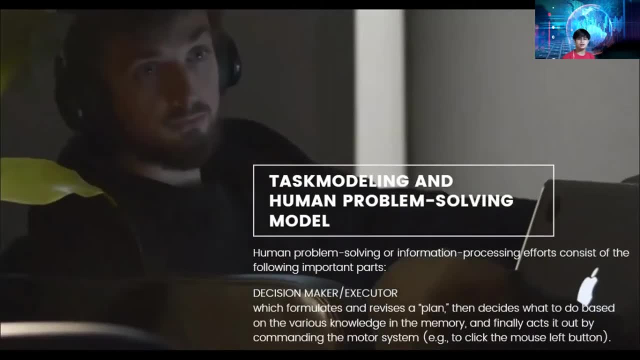 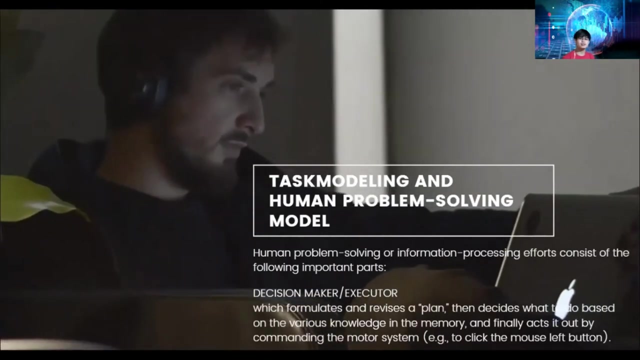 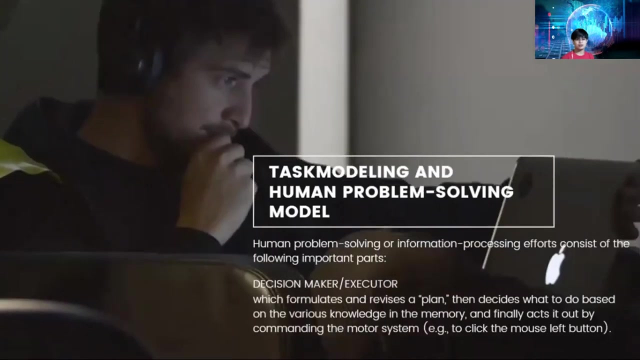 on the various knowledge in the memory and finally act it out by commanding the motor system. Okay, For example, Re-click the mouse left button or Right-click left button Or Right-click right button, Something like those things. Okay, So those were. how are you going to task modeling? that is the Task Modeling and Human Problem. 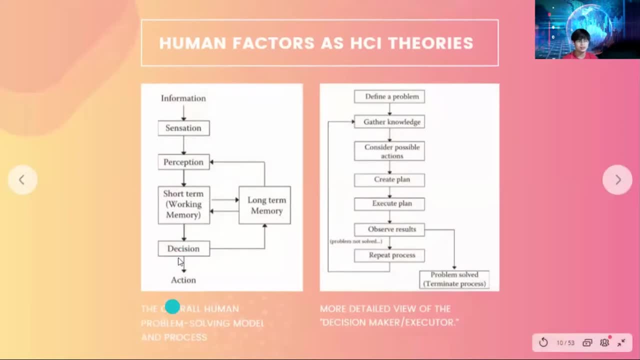 Solving Model. Okay, So here it is. This is the representation. Okay, Let's say there is an information. Okay, An information, it will run through the sensation And after the sensation, it will be sent to the task. 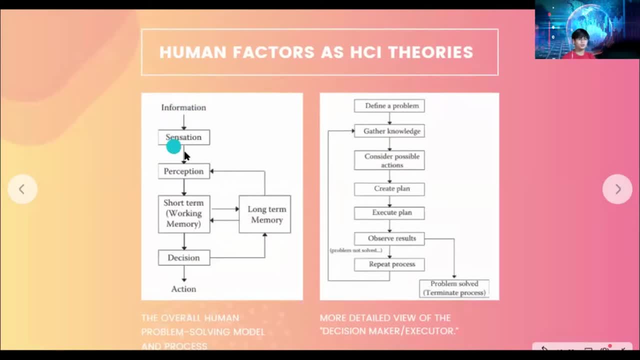 Okay, So that's the task, And the task is going to be sent to the human problem solving model. Okay, So here it is. This is the representation. Okay, It goes to the perception, Your perception, Okay. 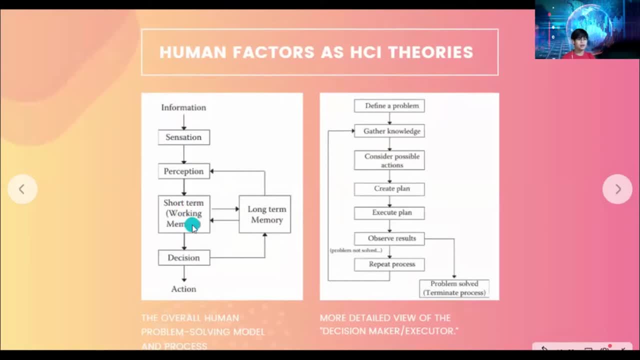 It goes to the memory, Right, It goes to the short-term memory And then it goes back and forth to the long-term. Okay, Then it will go to the perception, And then we're going to, you know, because of the perception, and then short-term, long-term. 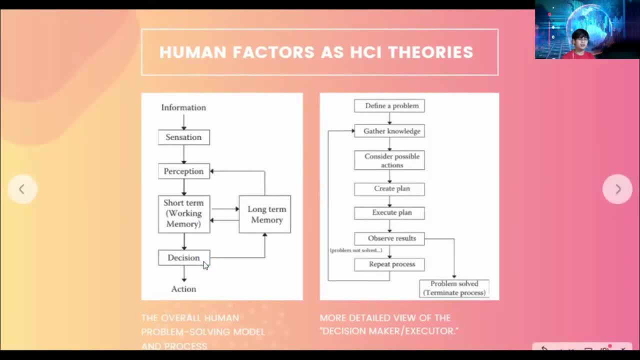 memory, then we're going to make a decision And after making a decision, of course, we take an action. Okay, So, this is the overall human problem solving model. in French, This is what can happen. Okay, So, for example, when I click an icon in the computer, I know in my Android phone: okay, 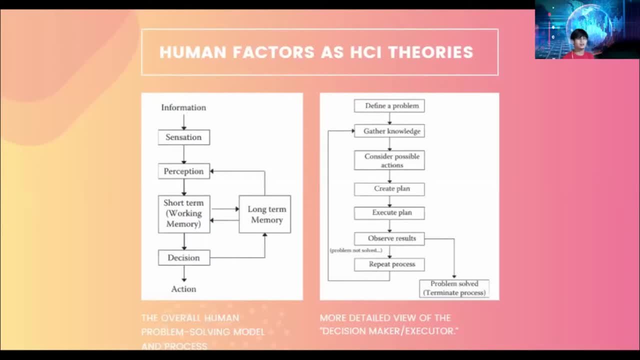 So there's a sensation, And then what is my perception? then The next thing that can happen. So we're going to store it in the memory. It's right there, And then I'm going to remember that one. 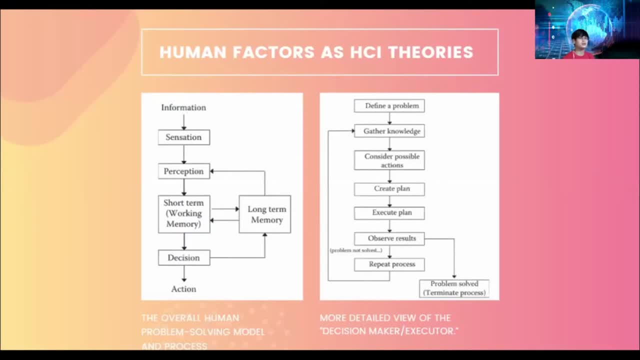 And then, of course, I decide you know to use after clicking the icon. Okay, So after clicking this button, the user will be navigated to this page, or etc. And then what will be the action? Okay, 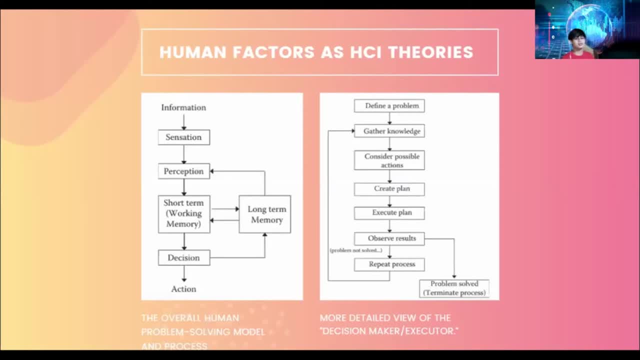 So that is again the overall problem solving model and process For the more detailed view of the decision maker or executor, of course, what you're going to do in order for you to model a task- or, yeah, you need to define the problem. 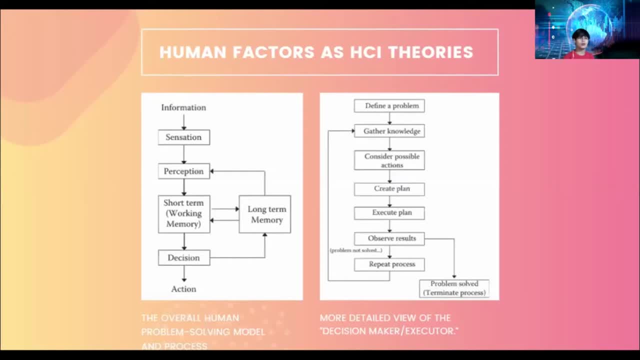 Okay, So, after defining the problem, you gather knowledge. Okay, The basic one. Okay, Consider possible actions. What will be the possible actions? Okay, You create a plan And then, after creating a plan, you execute, And then you observe the results. 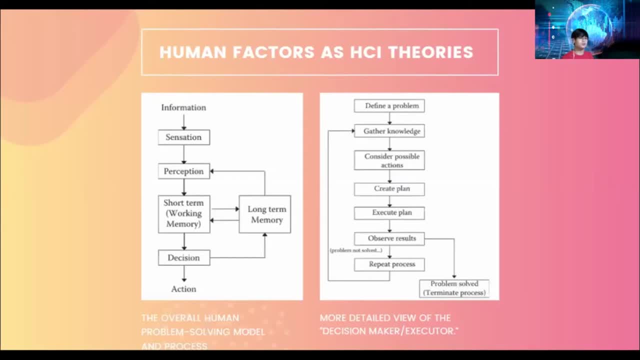 Okay, So if the problem is not solved, you go back to gathering the knowledge And then if, after observing the result, then the problem is solved, The process will be terminated. Okay, So, as easy as that. So a simple illustration would be insecurity. 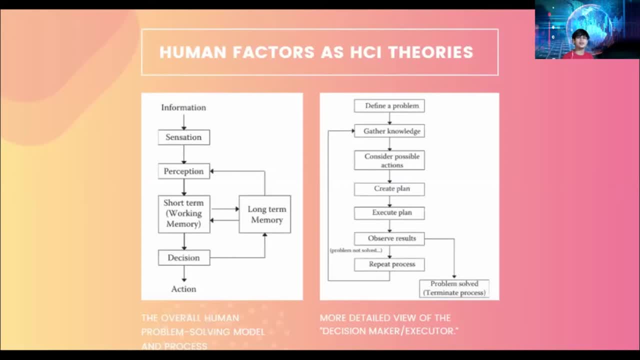 You know, The user will not be able to access the dashboard of your system without, you know, registering or plugging into the application. Okay, So what is the problem in there? The problem would be, if the login page is not there, then it will automatically access. 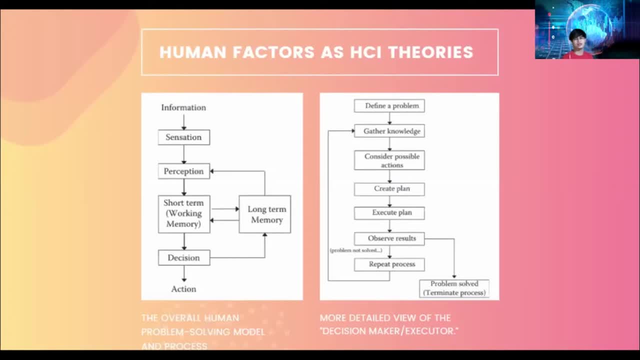 So what are you going to do? You need to create an interface with this. with that, Okay, So the user will be able to log in if the user's password is invalid. So, if not, what are you going to do so that they can log in? 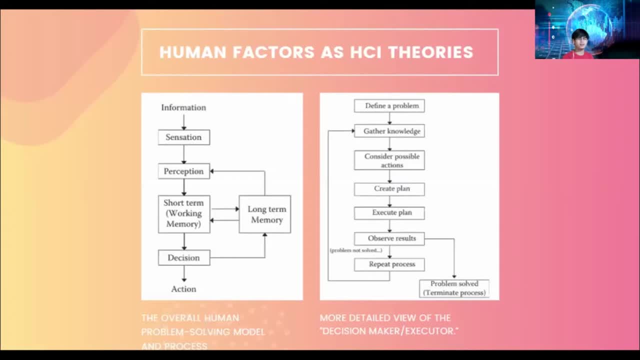 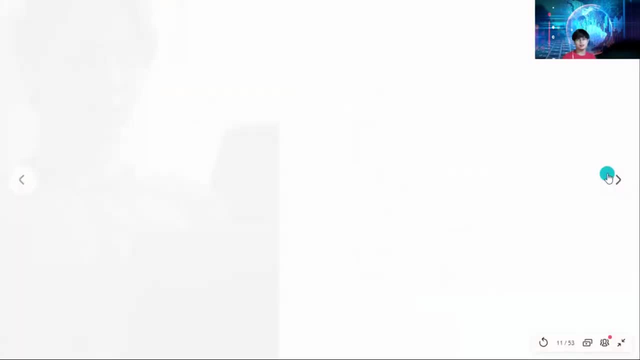 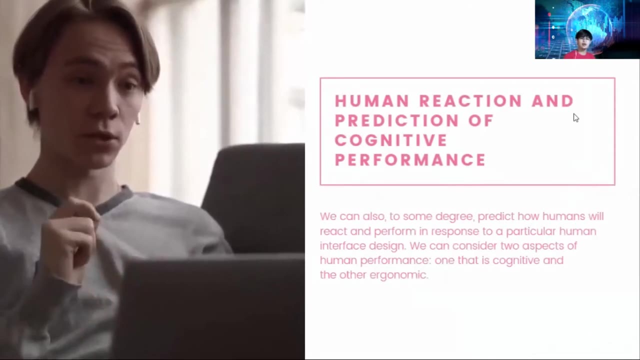 Okay, So those are some pretty basic illustrations for that, guys. Next Let's move on to human reaction and production of cognitive performance. Okay, We can also to some degree predict how humans will react and perform in response to a particular 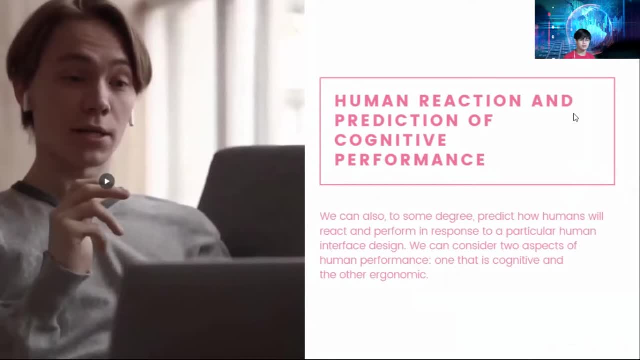 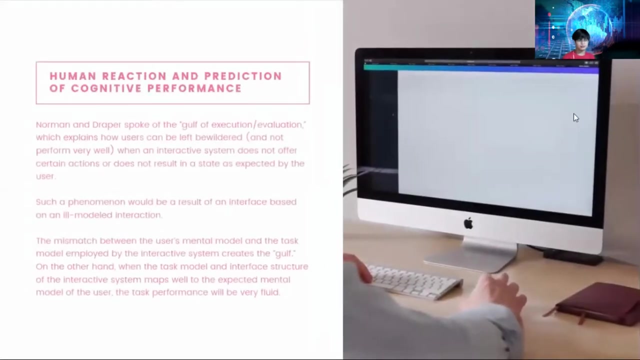 human interface design. This is really true And I absolutely agree with this one. So we can consider two aspects of human performance, One that is cognitive and other is ergonomic. Okay So, okay. So the human reaction and production of cognitive science. 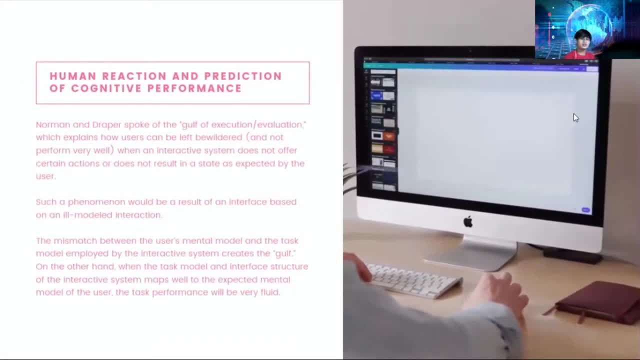 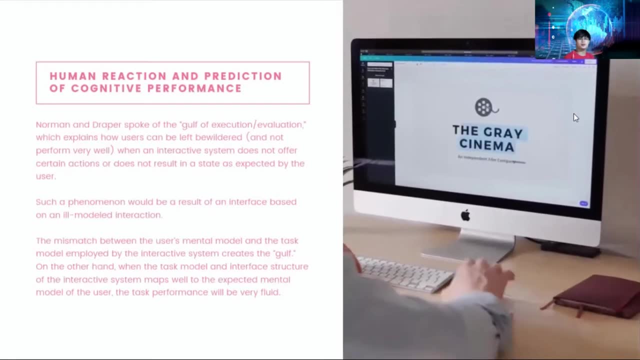 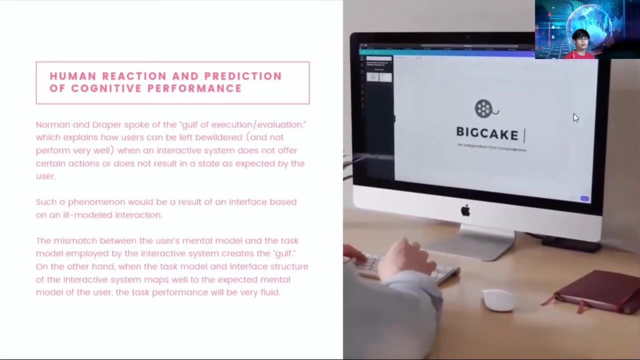 So what is this cognitive now? Okay, So Norman and Draper spoke of the goal of execution or evaluation, which explains how users can be left bewildered and not perform very well when an interactive system doesn't offer certain actions or does not result in a state as expected by the user. 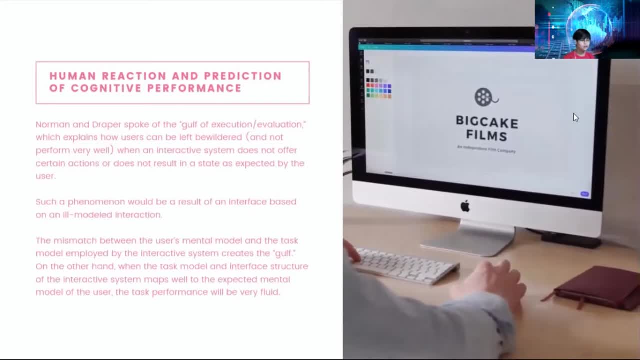 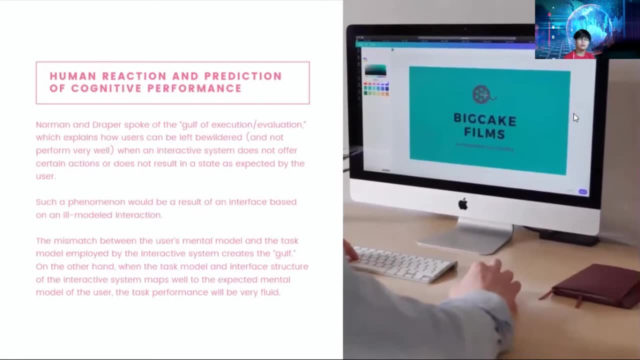 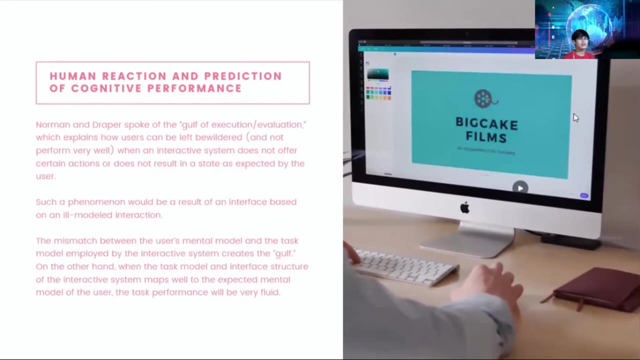 Of course, imagine: Okay, There's a button- register button- So it is expected If you click the register button you will be registered to the user, providing your name, your email, your phone number and etc. And then nothing will be seen. 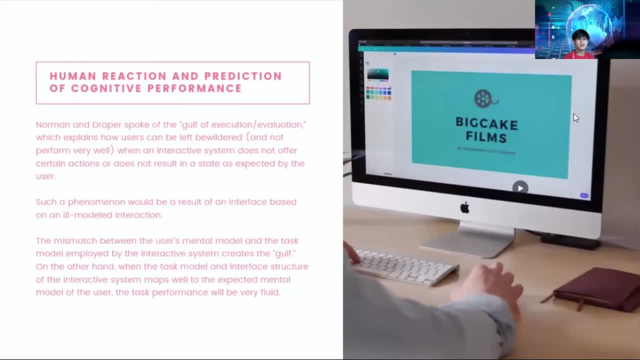 If you click the register button. Okay, So that is how you actually react, how you interact with the system. So such a phenomenon would be a result of an interface based on an L-modeled interaction. Okay, So if the user you know was not able to get the expected result, it will be again. 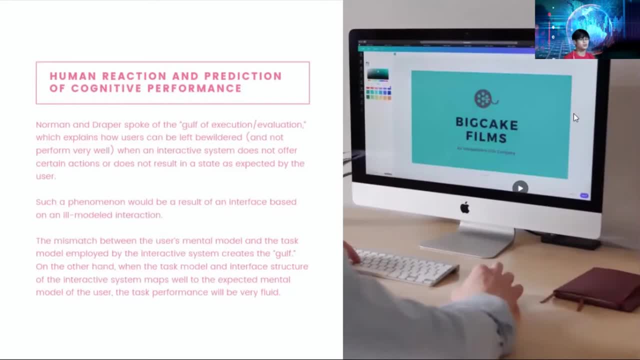 based on an L-modeled interaction. So it's very necessary, guys, that when you create a system, it should be modeled properly. Okay, The task must be defined properly and, yeah, should be planned out very well, Okay. 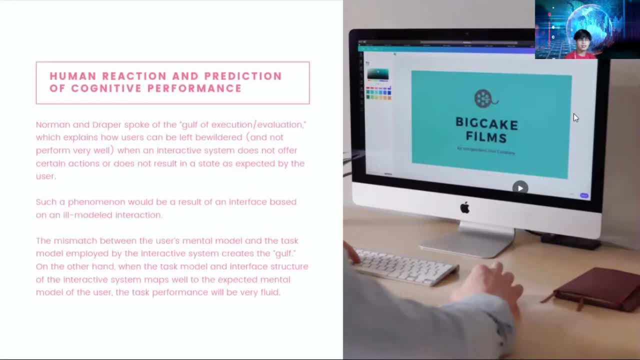 So the mismatch between the user's mental model and the task model employed by the user and the interactive system creates the goal Okay. On the other hand, when the task model and interface structure of the interactive system maps well to the expected general model of the user, the task performance will be very 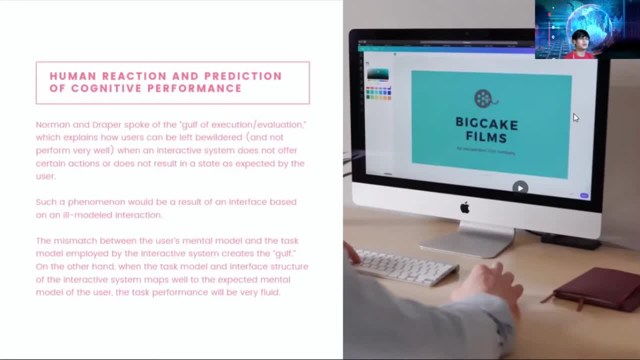 fluid. It's very necessary that when you create a system, you must predict you know what would be the expected output when the user uses this kind of feature, something like that. So it's all up to you, It's all your choice. 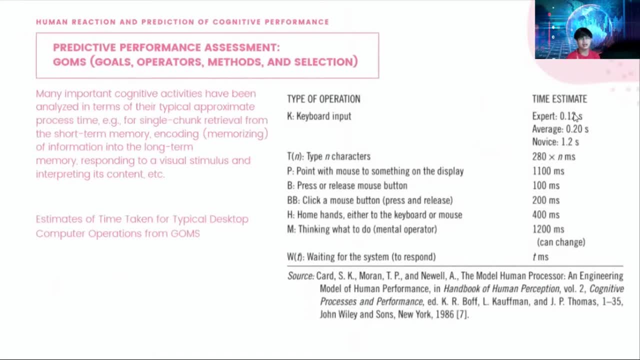 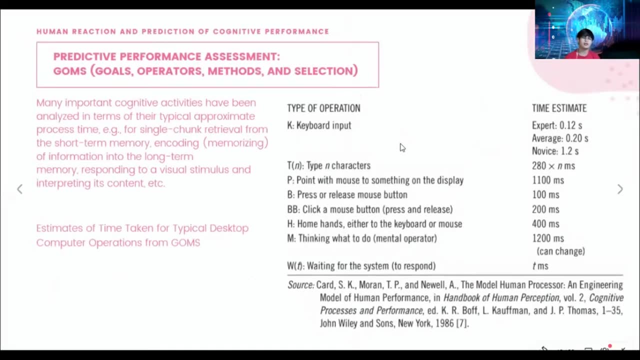 You need to plan it out, Okay, So just take a look at this one. This is the predictive performance assessment with GOMS, And GOMS meaning, goals, operators, methods and selection. Okay, So many important cognitive activities have been analyzed in terms of their typical approximate. 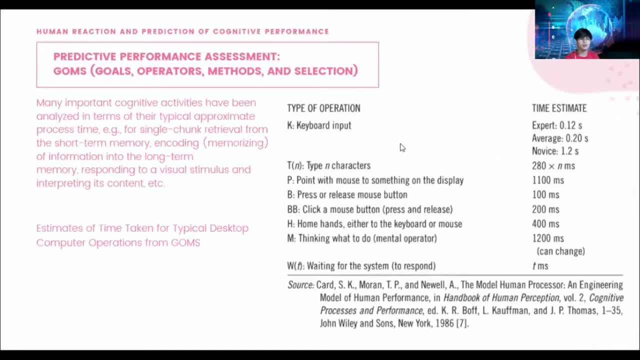 process time. So in terms of typical approximate process time, Okay. So for example, for single-channel retrieval from the short-term memory, encoding or memorizing of information into the long-term memory, responding to visual stimulus and interpreting its content and estimates of time for a typical list of computer operations from GOMS. 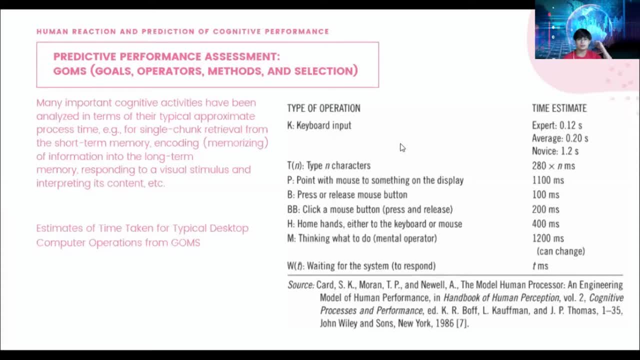 Okay. So for example, a keyboard input: Okay, The time estimate would be something like this: 0.2 seconds. or when a user points with mouse to something in the room: Okay, And the display You press or release mouse button. 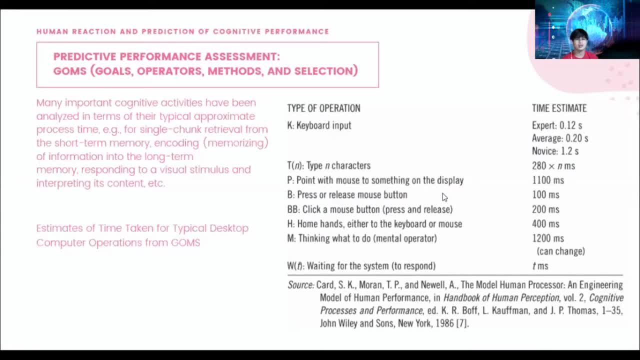 How many seconds will it take? You need to click a mouse. Home hands either the keyboard or mouse. Okay, So this is the predictive performance assessment with goals. So this is actually a sample. Okay, When you type in something in the computer. 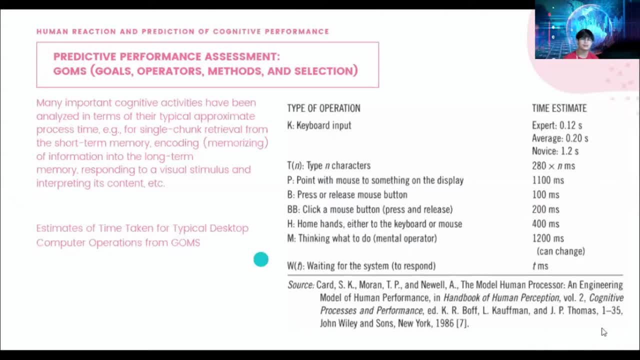 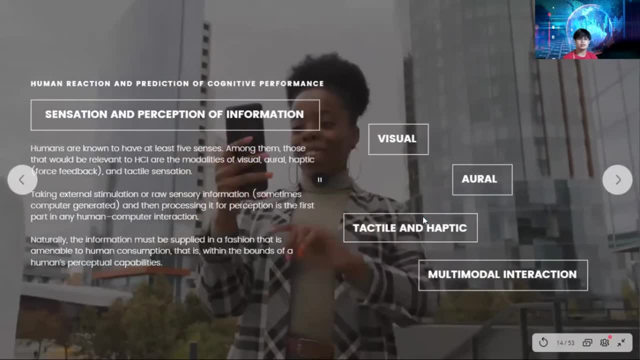 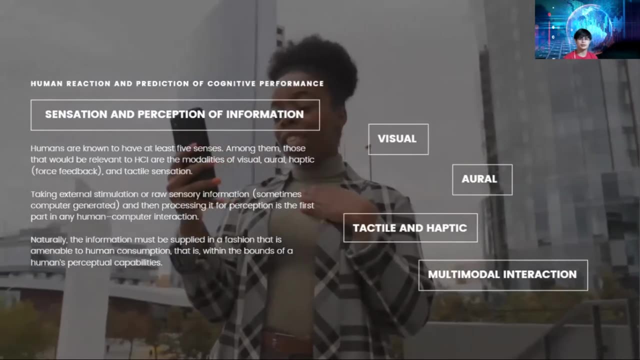 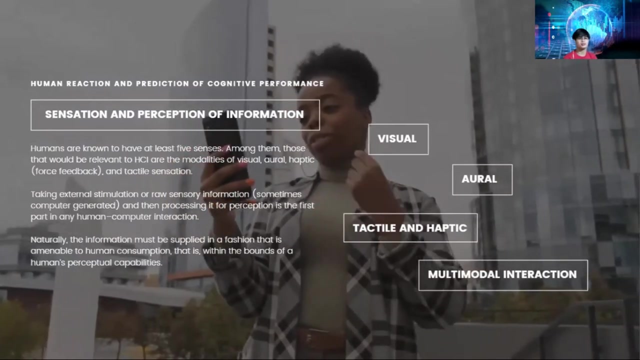 Okay, Okay, Next, Wait, Okay. Next that we're going to discuss would be the sensation and perception of information. Okay, So this is very important when you actually create a really good HCI design. So you must know the basic concept of sensation and perception of information. 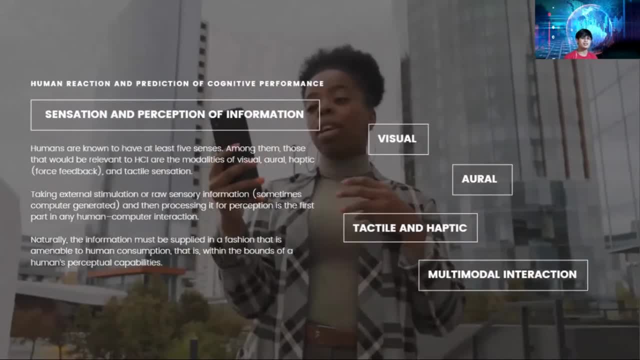 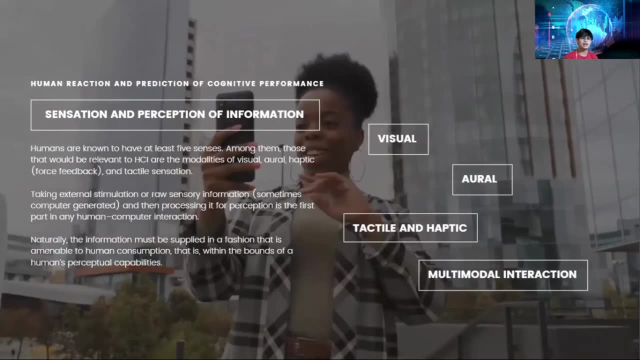 So humans are known to have at least five senses. Okay, So grade one is like this. Okay, So among them, those that would be relevant to HCI, are the modalities of visual. Of course we're using our eyes. 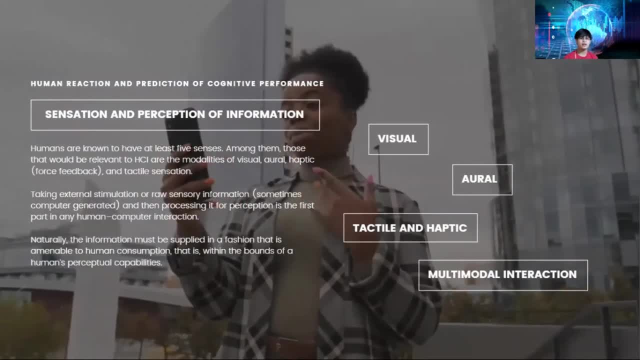 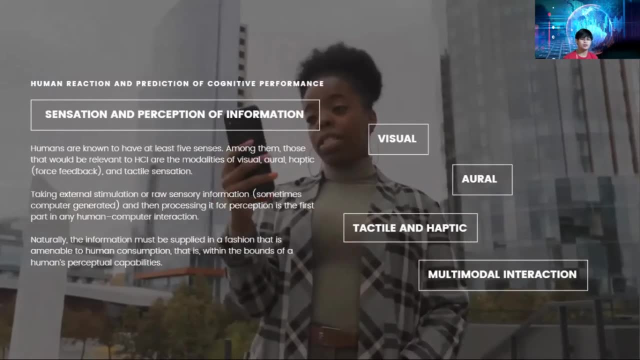 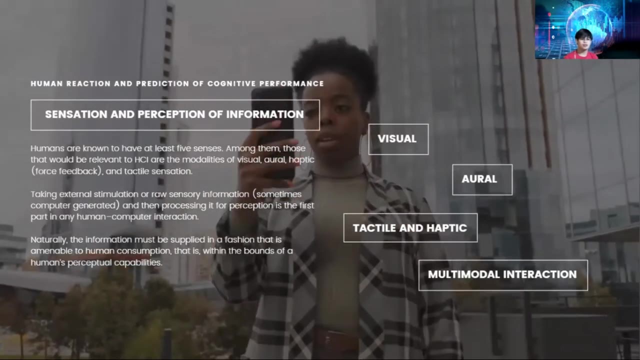 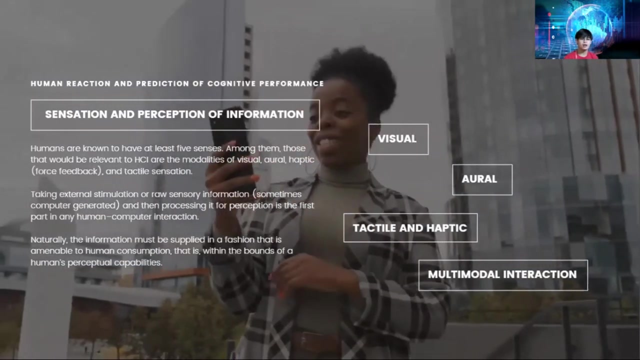 The oral, the hearing, the haptic or the touch, Of course, feedback and tactile sensation. Okay, So don't worry, because we're going to discuss each senses in the next slides. So taking external stimulation or raw sensory information, sometimes computer generated, 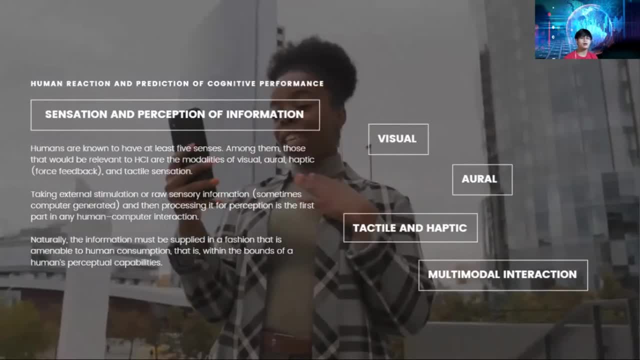 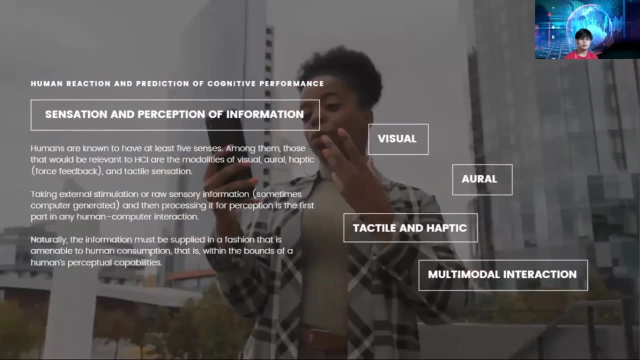 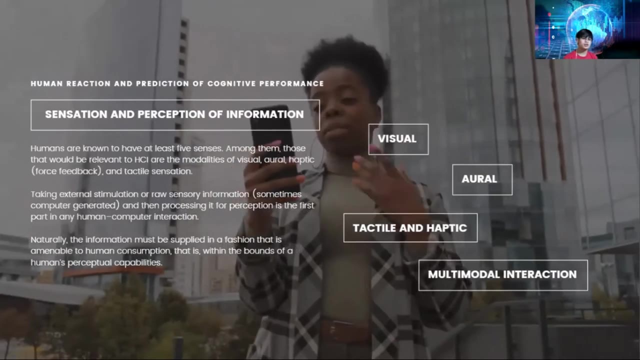 and then processing it for perception is the first part in any human computer interaction. Okay, So naturally the information must be supplied in a fashion that is amenable to human consumption, that is, within the bounds of a human's perceptual capabilities. So let's start. 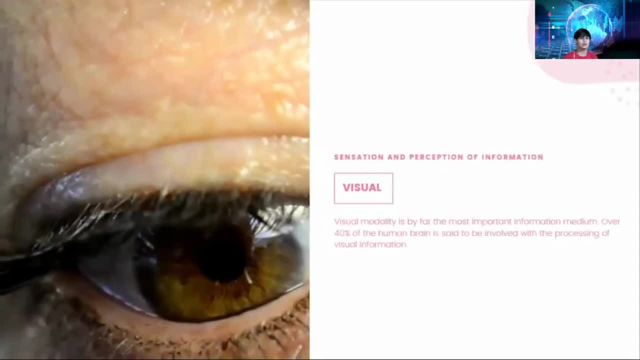 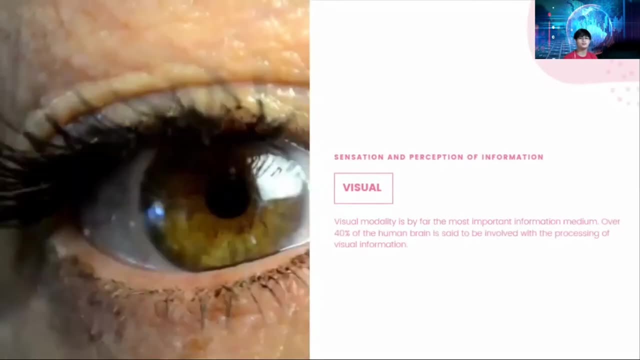 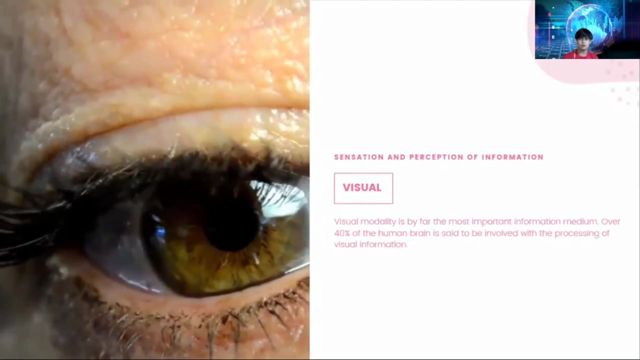 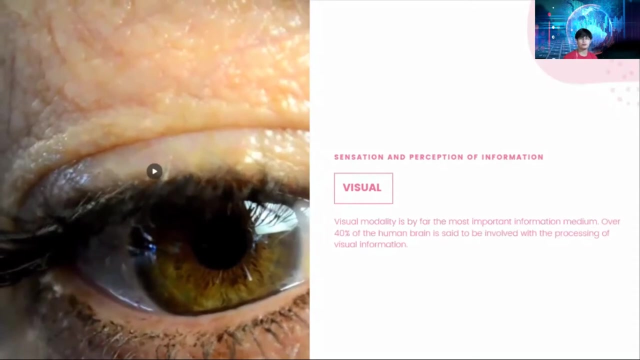 We're going to go with the visual. Okay, So visual modality is by far the most important information medium. Of course, how can you get the information if your eyes are closed? Okay, So we're going to discuss next with the sound, the information. 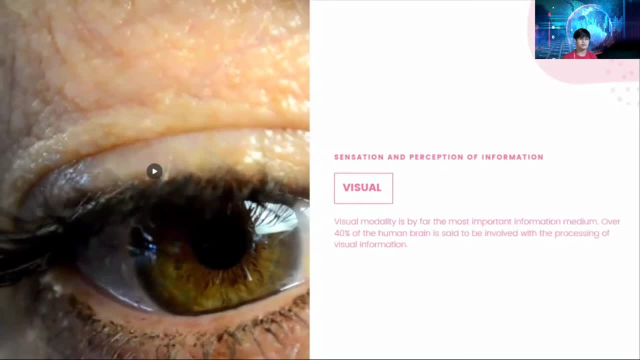 But for this slide, For this slide, it's very important. no, The visual modality is by far the most important information medium, So over 40% of the human brain is said to be involved with the processing of visual information through our eyes. 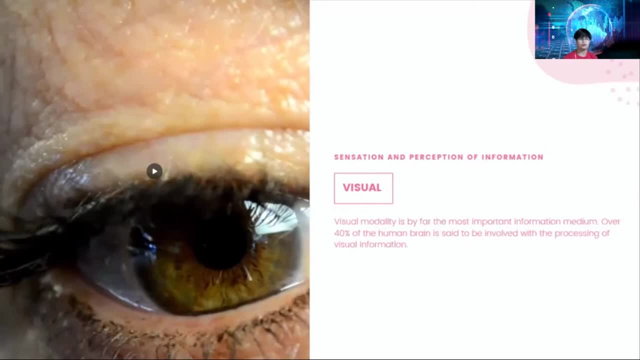 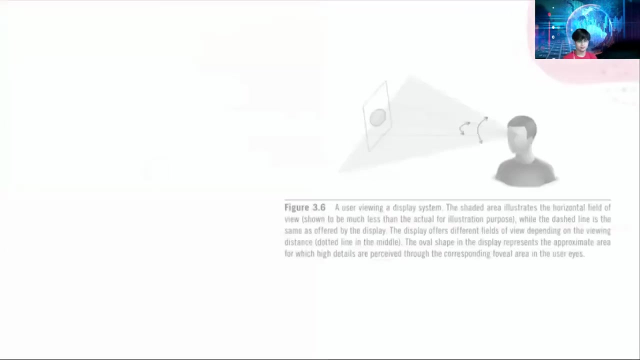 So again, it's over 40% of human brain. no, That's what we're going to use. It's easier to calculate. It's easier to calculate, of course, create over information through our eyes. Okay, So in visual we have this: visual and display parameters. 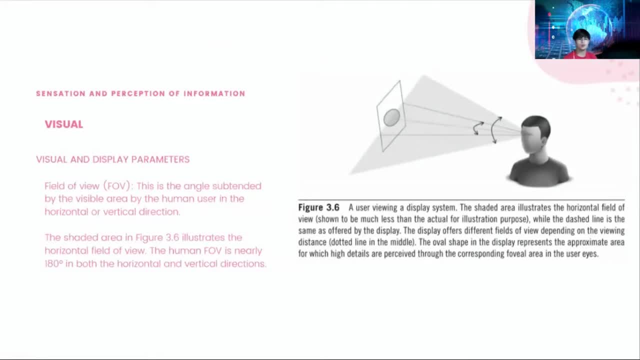 Okay, So first is the field of view. So the field of view or FOB. this is the angle subtended by the visible area, with the human user in the horizontal area. Okay So, as you can see in the image, the shaded area illustrates the horizontal view. 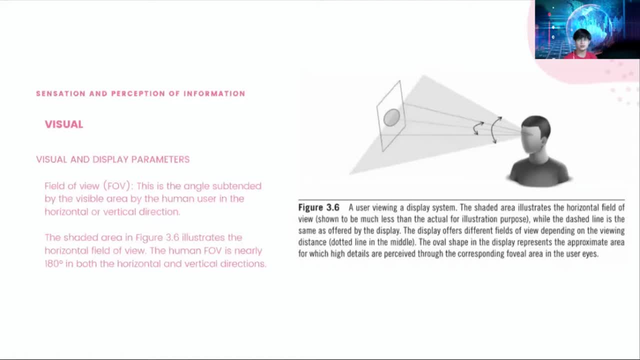 Okay So the human field of view is nearly 180 degree in both the horizontal and vertical direction. Okay So, as you can see in the figure, a user viewing a display system. So this is sample, not only display system. 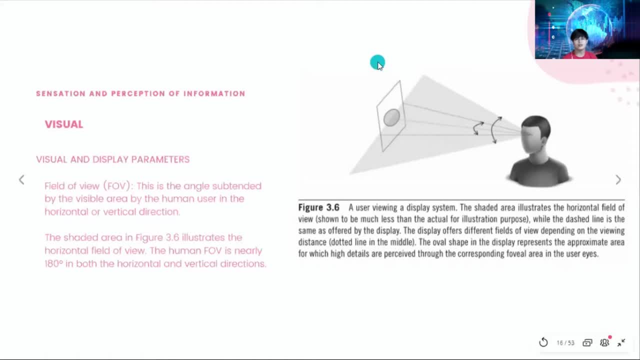 The shaded area illustrates the horizontal view: Okay. The shaded area illustrates the horizontal field of the view: Okay. Shown to be much less than the actual for illustration purpose. This is just an illustration purpose, So, while the dashed line is the same as offered by the display, 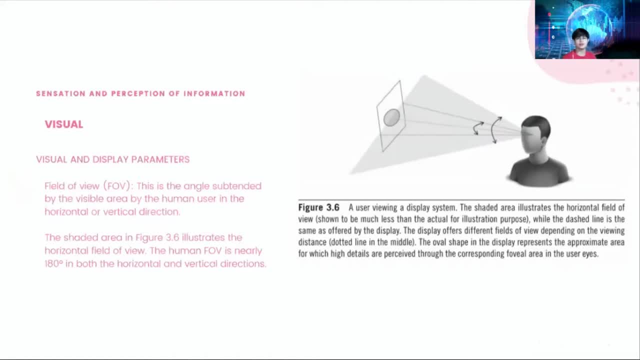 Okay. So the display offers different fields of view depending on the viewing distance. That is the line in the middle, As you can see here. this is the dotted lines. Okay. So the oval shape? Okay, The oval shape in the display represents approximate area for which high details are. 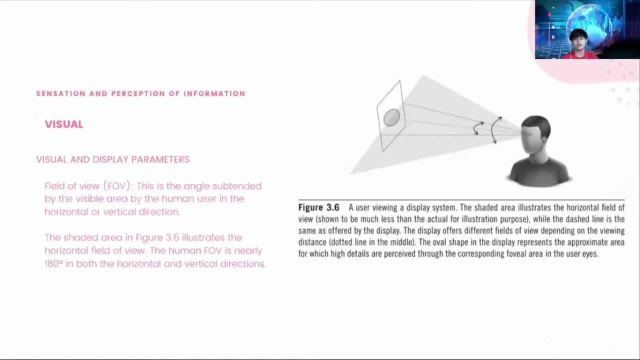 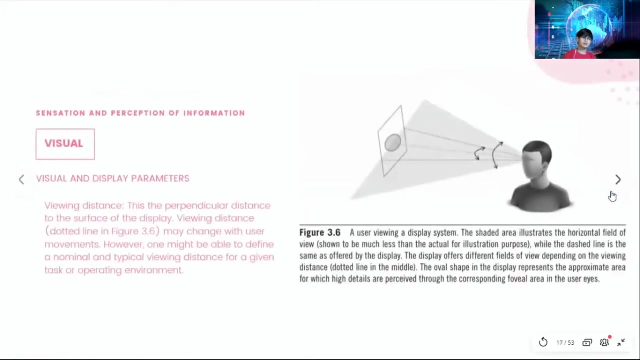 perceived through the corresponding oval area in the user eyes. Okay, So this is the sample. Okay, So again, there is a field of view when it comes to the visual and display parameters. Okay, Next is the viewing distance, So how the users view. 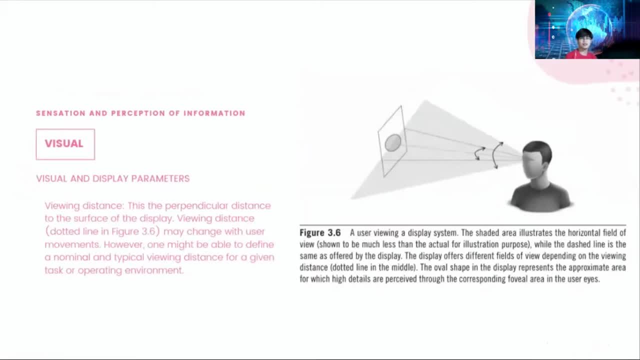 This is the distance given by the device, the eye. Okay, So the viewing distance. So this is perpendicular distance to the surface of the display. Okay, Again, a perpendicular distance to the surface of the display: Viewing distance. as you can see here the dotted lines, 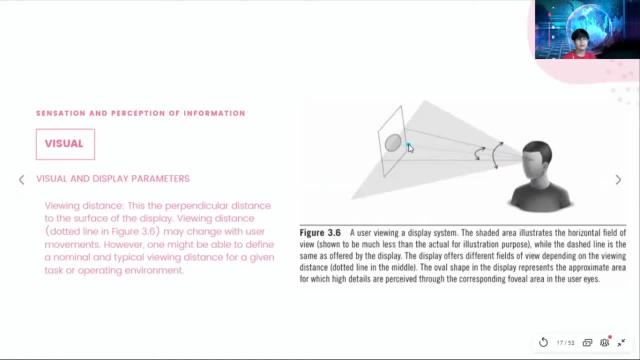 This is the viewing distance May change with user movements. You may have observed, You may notice that you are looking at it right. okay so. however, one might be able to define a nominal and typical viewing distance for a given task or operating environment. okay, so there's a viewing. 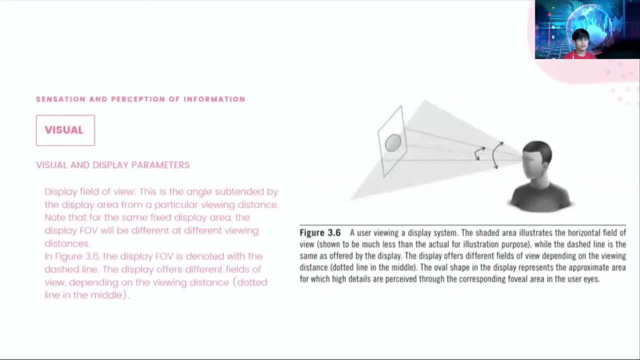 distance. next, also in a, in a visual display parameters, there is a display field of view. so again, please do not, do not be, I know, don't ask yourself an autonomous anymore when this does. we need to know this, we need to know the basic concepts, okay, in order for you to develop a really good design and then 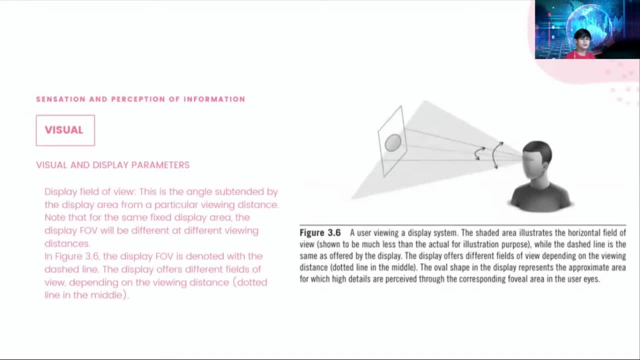 display field of view. in the display field of view, when it comes to the visual and display parameters, this is the angle subtended with the display area from a particular viewing distance. okay, so note that for the same fixed field display area, the display, if OB, will be different at a different viewing. 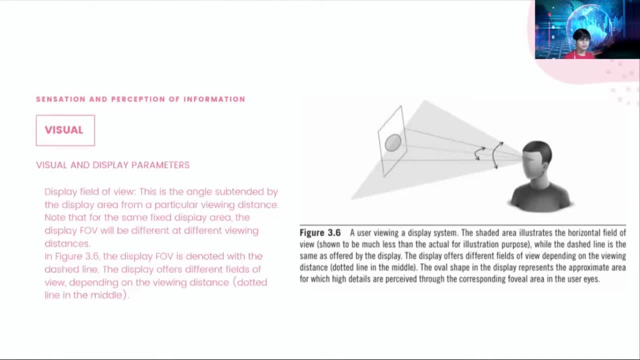 distance. so again in the figure 3.6, the display fob is denoted with the dashed line. dashed line, so the displays offers different fields of view depending on the viewing distance, or that in line in the middle. okay, so that is the display field of view. next is the pixel. the pixel is a display. 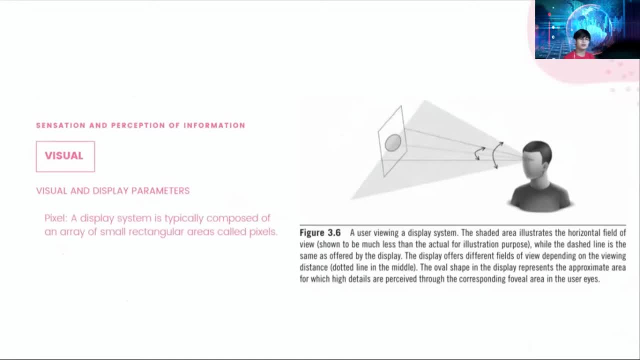 system. a display system is typically composed of an array of small rectangular areas called pixels. so if you are familiar with this, you can see on your screen it is, of course, composed with different pixels that will make it, as you know, I know, square. so I I believe you are familiar with this. 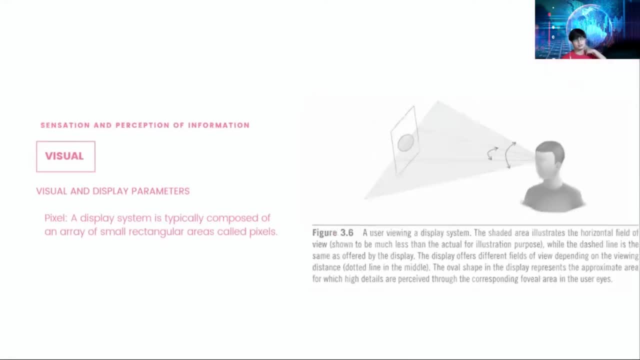 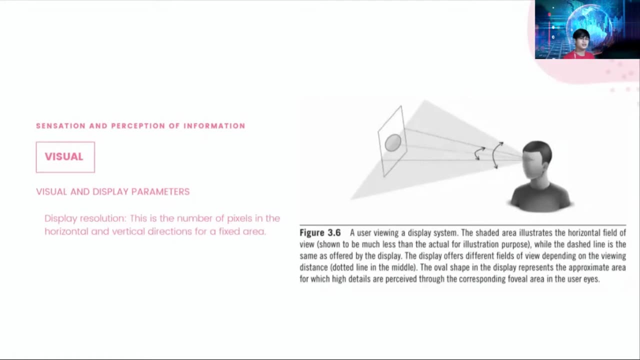 cabrón amana: pixels. okay, the display resolution. so when you design, you need to know from. for a person. okay, you need to know the display. different display resolutions. so, as we have observed that in our laptops, not in our smartphones, only my different resolutions. tablets: okay, so this is the number of pixels in the horizontal and. 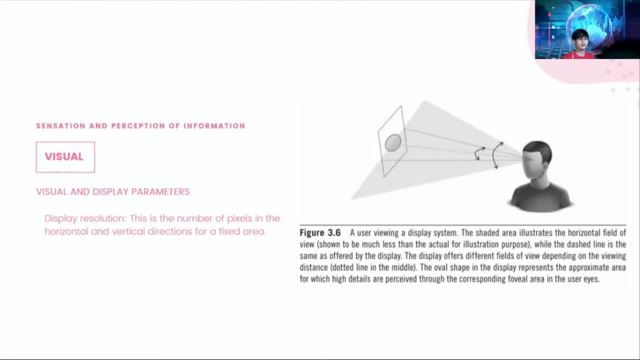 vertical directions of a fixed area. okay, that, it's just a basic one. the visual, accurate. okay, the visual activity and effect: this is the resolution per second resolution perceivable by the human eye from a fixed distance. okay, this is also synonymous with the power of sight, which is different for different people in each. 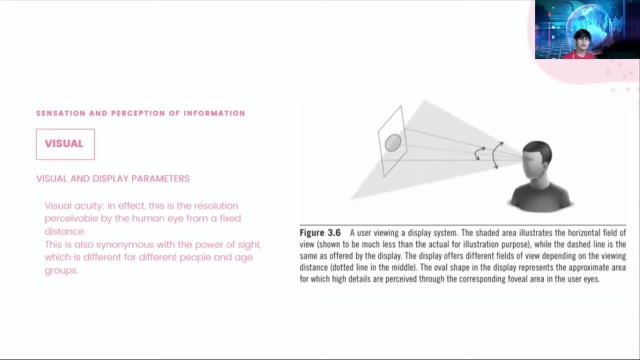 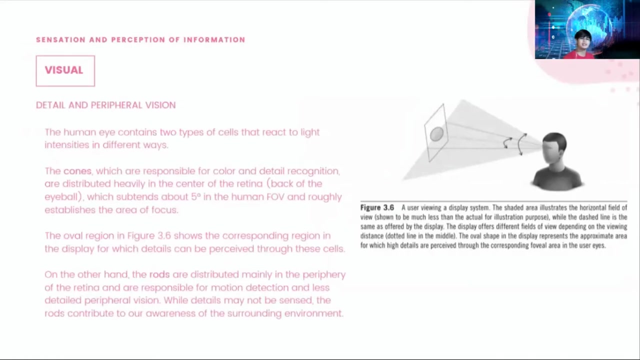 group. okay, again, this is just the resolution perceivable by the human eye from a fixed distance. that is, the visual activity. okay. next, when it comes to the visual, is the detail and peripheral vision. okay, so the human eye contains two types of cells that react to the light. 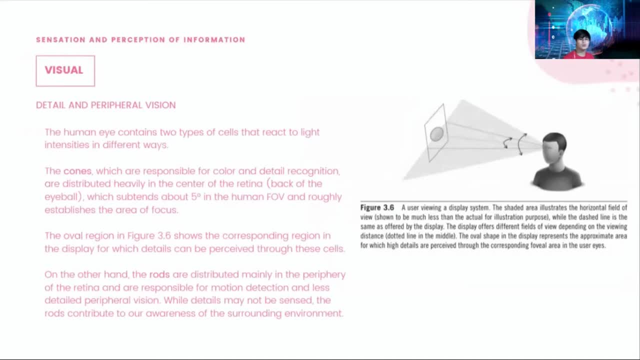 intensities in different ways. the cones which are responsible for color and their recognition are distributed heavily in the center of the retina, back arm of the eyeball, which subtends about five degree in the human FOB or field of view and roughly establishes the area of vocal. okay, so the oval region in 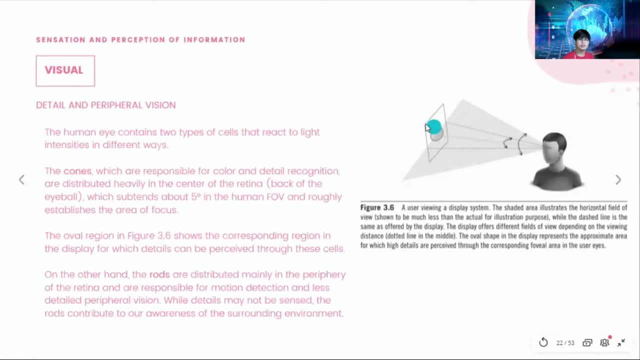 0.6, as you can see in here, shows the corresponding region in the display for which details can be perceived through these cells. so, on the other hand, the rods are distributed mainly in the periphery of the retina and are responsible for motion detection and less detailed peripheral vision. 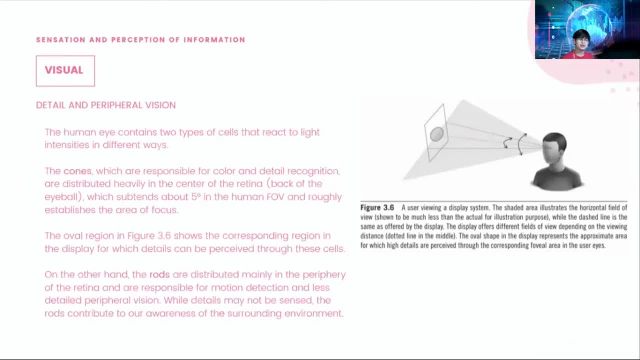 so, which details may not be, sense, the rods contribute to our awareness of the surrounding environment. so, um, this is just concept in you know, image, imagine, but we're not gonna, you know, um, explain further. all you have just to do is there is, uh, two types of cells that react to the light intensity. 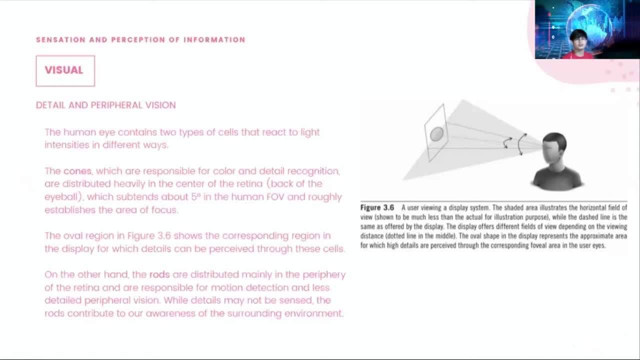 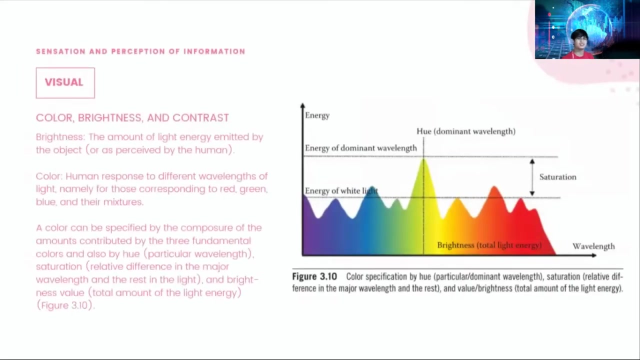 the cons and then the rats. okay, so if you wanted to learn more about how our eyes work, then study the other field you know of. you know studying the human eye. next, the color, brightness and contrast. I believe, because you're always you know photos, in your there is a really good brightness, no more contrast. 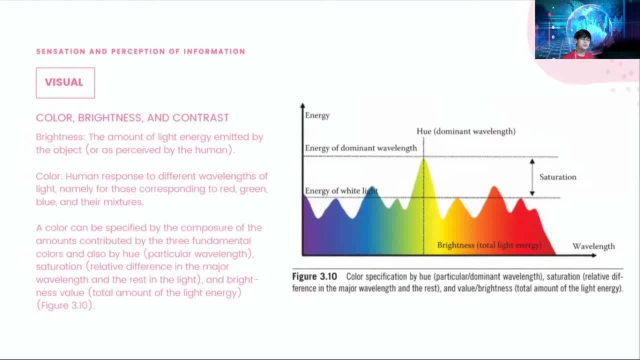 okay. so when we see brightness again, the amount of light energy emitted by the object, the brightness, the color human responds to different wavelengths of light, namely for those corresponding to red, green, blue and barometers. that is the color. okay, so a color can be specified by the composer composure of the amounts contributed by the three fundamental. 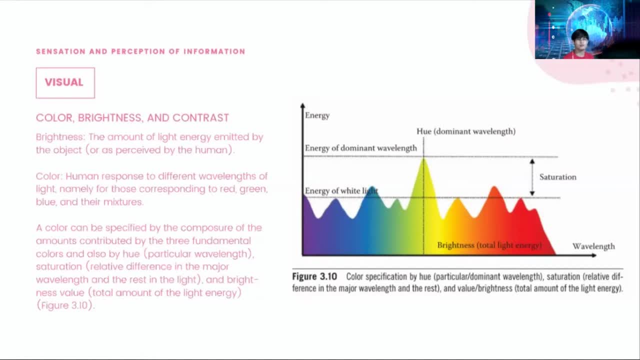 colors, and also by you or the particular wavelength. the saturation: okay, the saturation meaning the relative difference in the major wavelength and the rest of in the light and brightness value for the total of the light energy. okay, so this is a sample. uh, this is the figure in three figures: 3.10. 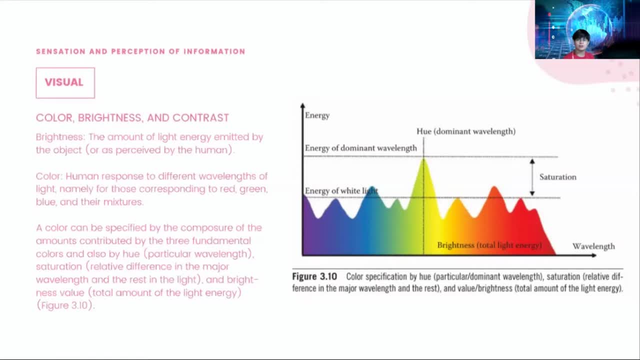 the color specification that you for particular, with dominant wavelength, with saturation again, is the relative difference in the major wavelength and the rest, and the value or brightness. this is the total amount of light energy. okay, so if you're going to use Lightroom, you know when you edit a photo. 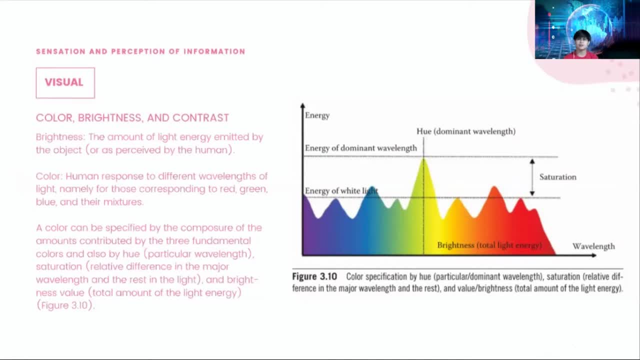 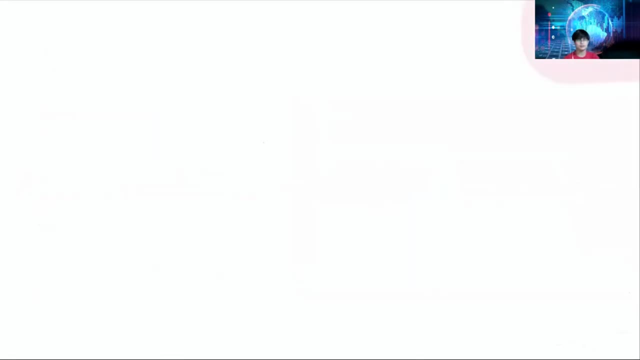 here. if you're adjusting the brightness, you add the colors in contrast, something like that. okay. so again, when you develop the system, you need to consider the color, the brightness, and then it's contrast, next the, the contrast. okay, the contrast, by the way, is this is the relative difference in. 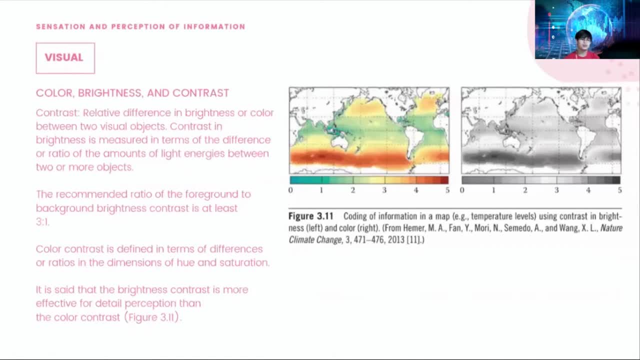 brightness or color between two visual objects. so contrast in brightness is measured in terms of the difference or ratio of the amount of light energies between two or more objects. okay, so the recommended ratio of the foreground to background brightness contrast is at least three of one. okay, then the color contrast is defined in terms of differences or ratios in the dimensions of you. 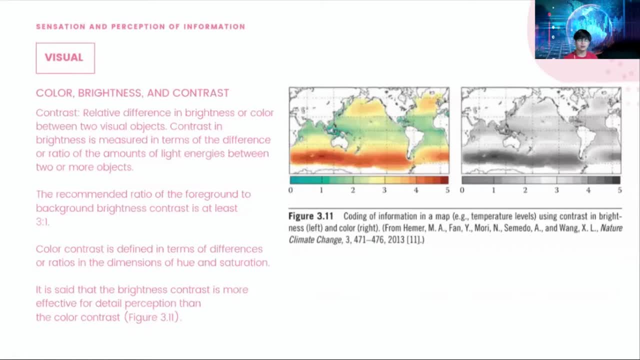 and saturation. so it is said that the brightness contrast is more effective of for a data perception than the color contrast. okay, so, as you may have observed, coding of information in the map, okay, using contrast and brightness left and then using the color in the right. okay. so, um, I believe and I hope you guys have already an idea, you know how contrast works. 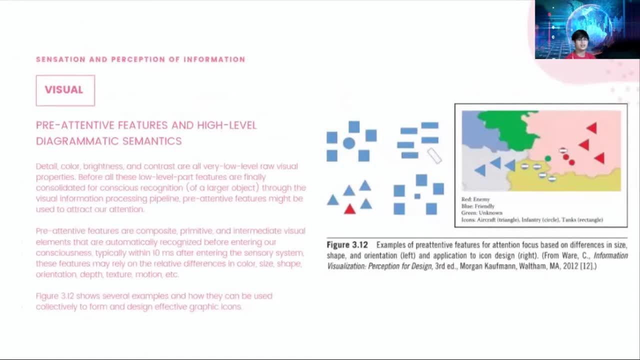 next, the pre-attended features and high-level diagrammatic semantics. okay, so, detail: I'm gonna show you guys the pre-attended features and high-level diagrammatic semantics. okay, so, pre-attended features and high-level diagrammatic semantics. okay, so, for example, for example, this: 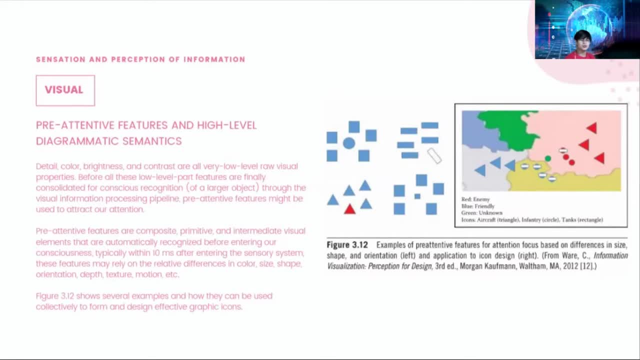 pre-attended features and high-level diagrammatic semantics. okay, so you can see that this is a very low level of low visual properties, and contrast and color brightness and contrast are all very low level row visual properties. so before all these low level part features are finally consolidated for conscious recognition of a larger object through the visual information processing pipeline, pre-attended features might be used to attract our attention. okay, wait, um. so how about this? 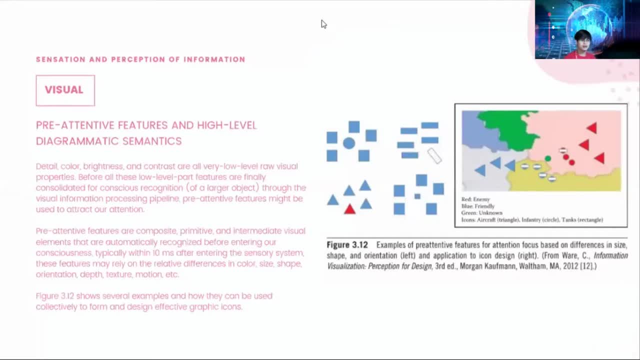 So what are these pre-identity features? Pre-identity features are composite, primitive and intermediate visual elements that are automatically recognized before entering our consciousness, So typically within 10 milliseconds after entering the sensory system. these features may rely on relative difference in color, size, shape, orientation, depth, texture. 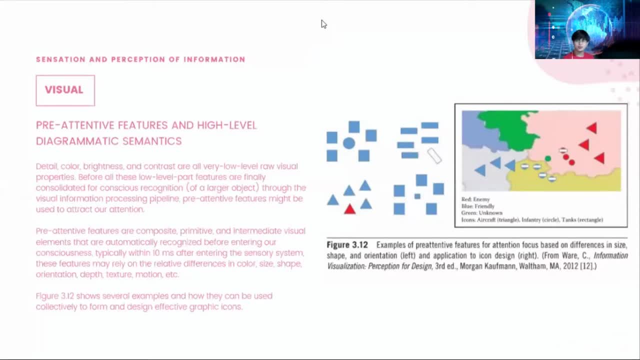 motion, etc. Okay, so, as you can see here in the chapter 12, this is just an example. This is an example of pre-identity features for attention focus based on differences in size, shape and orientation, and application to icon design in the right. 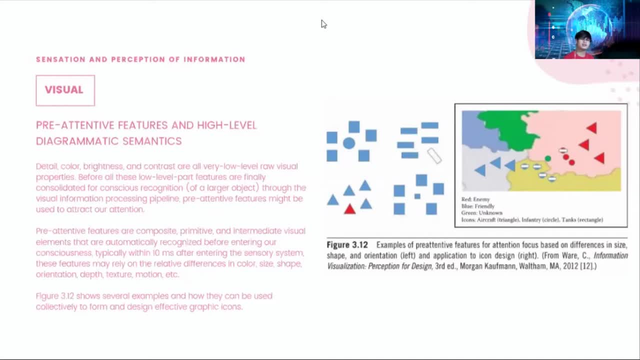 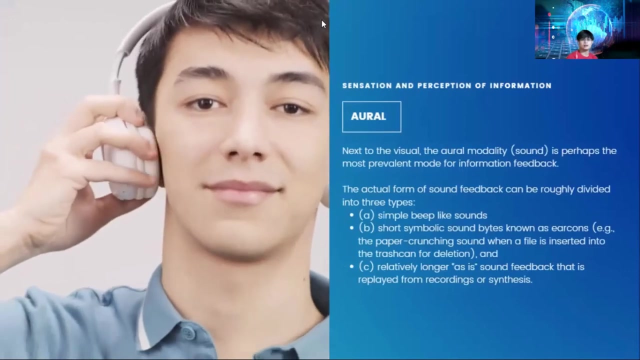 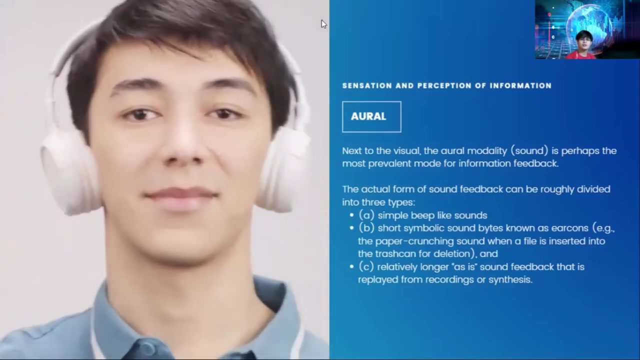 So, again, you're familiar with the different icons, yeah, that you can use when you actually create your ancestors. Okay. Next is the aural. okay, So next to the visual, the aural modality, or the sound, is perhaps the most prevalent. 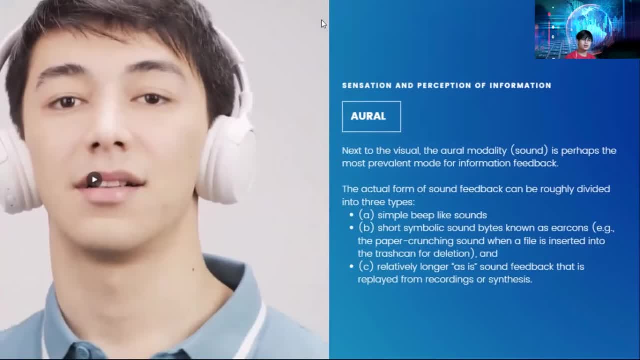 mode for information feedback. So again, um naay-uban sa tuwan ng mga users na possible dito sila kakita diba. they're blind, So how they actually get the information, It's through their ear, no. 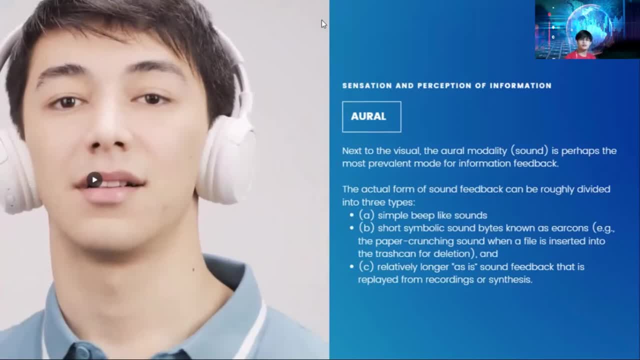 Okay, It's through sound. So the actual form of sound feedback can be roughly divided into three types: Simple beep-like sound. short symbolic sound bites, known as the earcons, The paper. an example for that would be the paper-crunching sound when a file is inserted. 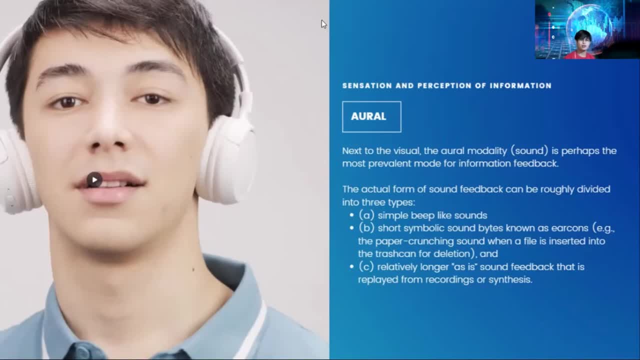 into the trash can for deletion. Kabalo kung naka-down naman alam, when you drop something to the recycle bin, mag-power up din siya diba Kung di mo bagay siyang i-delete, something like that. 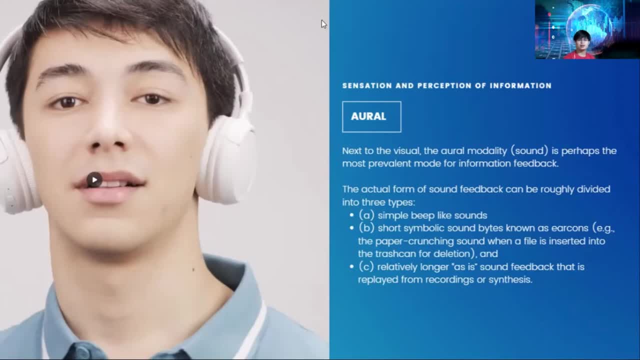 And then you know you can also use it as a filter. And then the relatively longer as is sound feedback that is replayed from recording or synthesis. Okay, again, the actual form of sound feedback can be divided into three types. 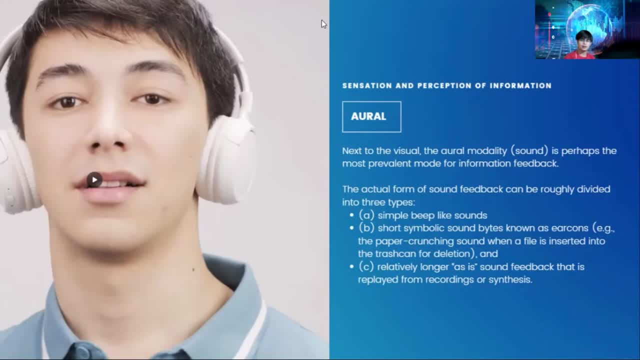 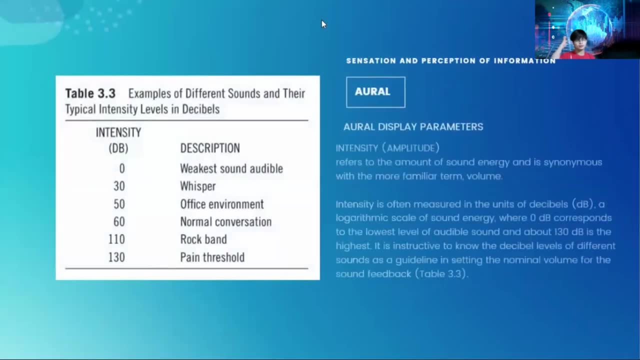 We have simple beep, short, symbolic and relatively longer, as is sound feedback that is replayed from recording or synthesis. Okay, so let's discuss the different oral display parameters. The first is the intensity, or amplitude. okay, It refers to the amount of sound energy and is synonymous with a more familiar term: volume. 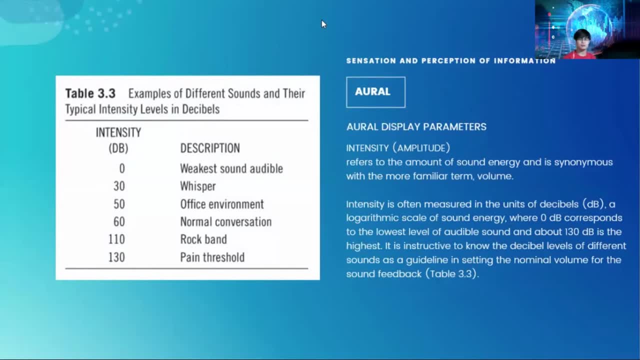 Okay, kabalo man tag ngayon mga volume diba. Pwede mo kita magpa-music. no, there's a volume, okay. Intensity is often measured in the units of decibels or dB, so a logarithmic scale of 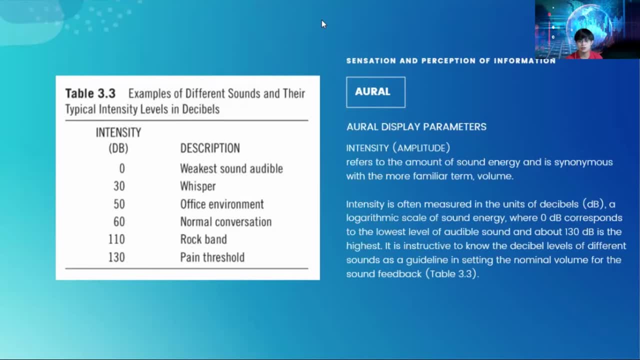 sound energy. Where is zero? Zero? the dB corresponds to the lowest level of audible sound in about 130 decibels is the highest. Okay, So it is constructed to know that the decibels of different sounds as a guideline in setting. 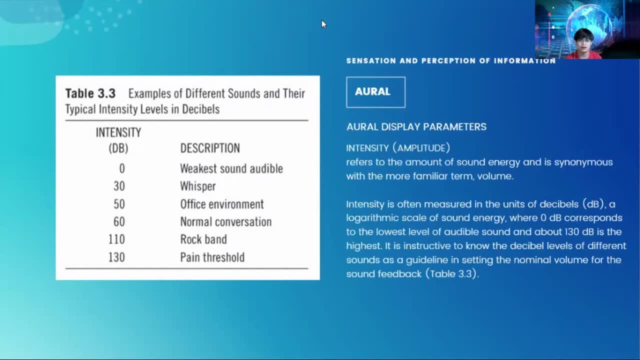 the nominal volume for the sound feedback: Okay, so the zero is the weakest, wala na no 30,. the whisper 50 is the office environment: Okay, The normal conversation: 60,. that is intensity. The rock band just 110, and then again the highest is 130,. this is the pain threshold. 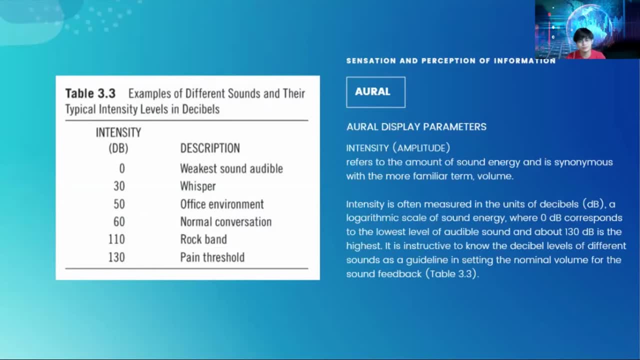 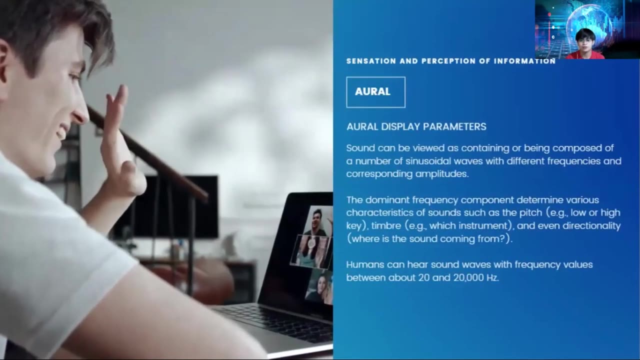 no, Siyang ke-100% na nila. no, Okay. So again, that is when we are talking about the oral display parameters or the sound. Next is okay. Sound can be viewed as continuous. Sound can be viewed as containing or being composed of a number of sensoidal waves, with 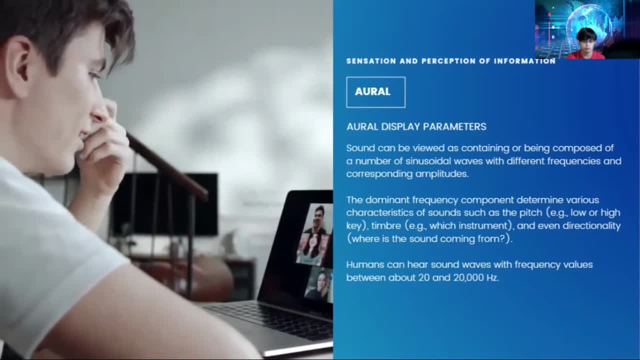 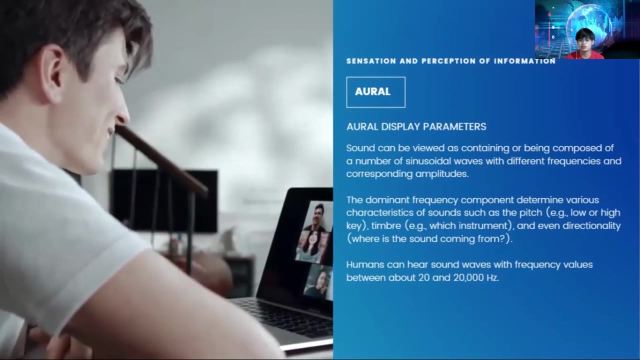 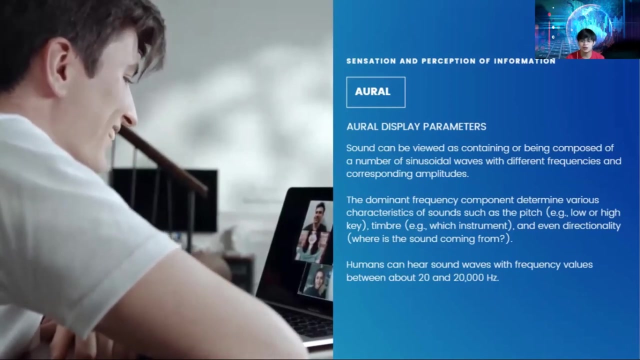 different frequencies and corresponding amplitudes. The dominant frequency component determine various characteristics of sound, such as pitch, low or high timbre. no, Which is the instrument? and event directionality: directionality: where is the sound coming from? So humans can hear, or can hear sound waves with frequency values between about 20 and 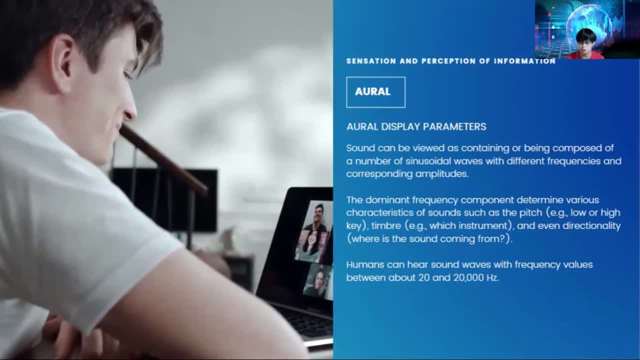 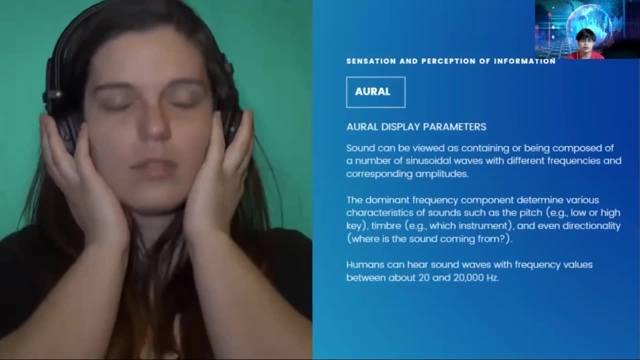 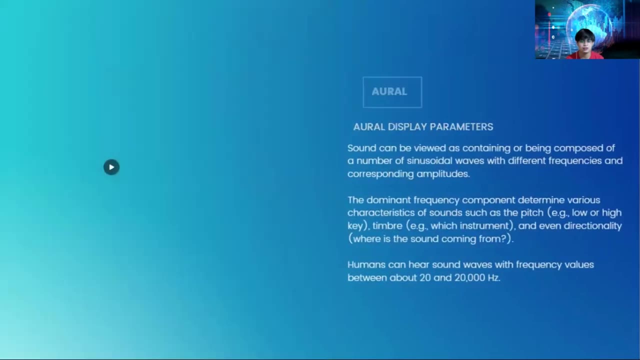 20,000 hertz. Just get a simple concept, okay, on how we actually hear. Oh, I think. okay, it's the same slides, so let's move on to the next: the face. Okay, The face. 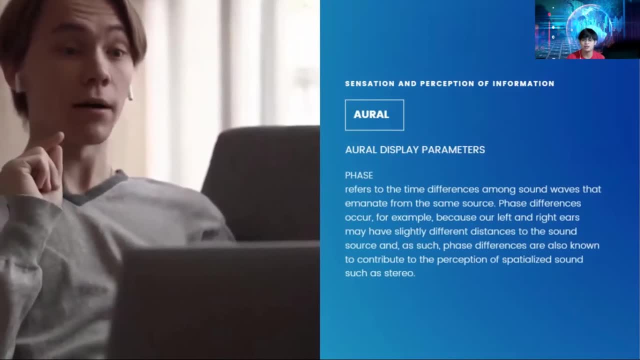 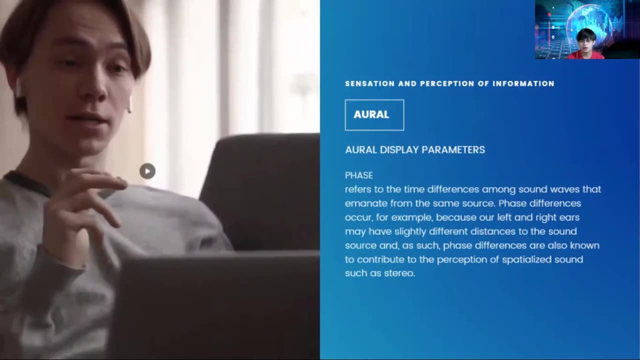 It refers to the time differences among sound waves that emanate from the same source. So face differences occur, for example, because our left and right ears may have slightly different distances to the sound sound source and as such, face differences are also known. 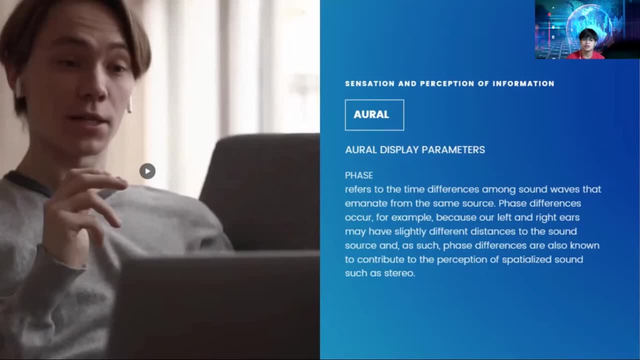 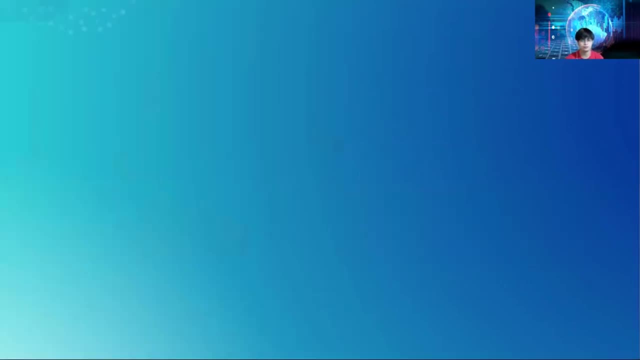 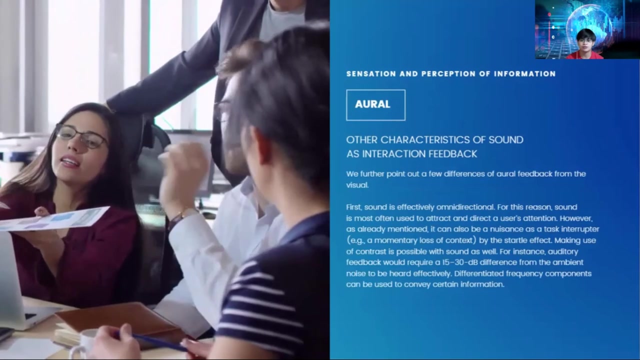 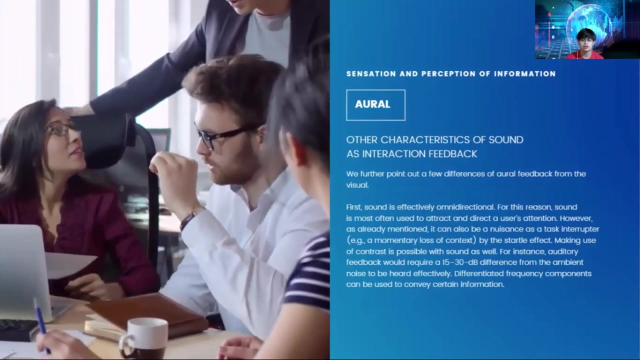 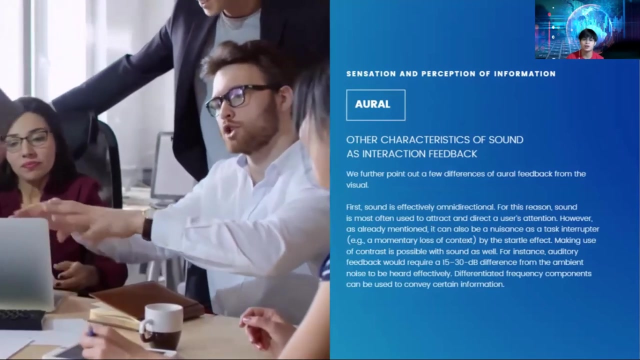 to contribute the perception of specialized sound such as stereo. Okay, Okay, Next is other characteristics. We further point out a few different ororal feedback from the visual. So first, sound is effectively omnidirectional. okay, So for this reason, sound is most often used to attract and direct a user's attention. 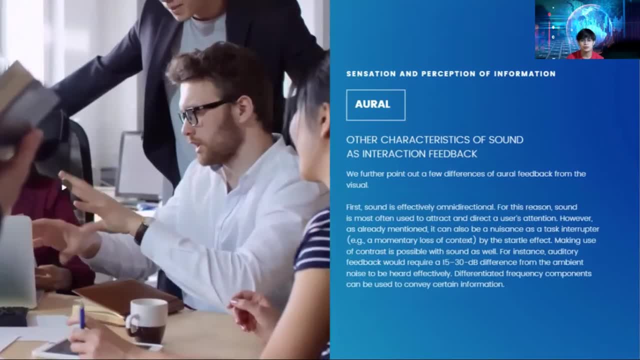 Okay. However, it's already mentioned- it can also be a noisance-attracted Here. first feature is sound reactions. Right, a test in interrupter. okay, for example, a momentary loss of context by the sterile effect. making use of contrast is possible with sound as well. for instance, auditory feedback would require. 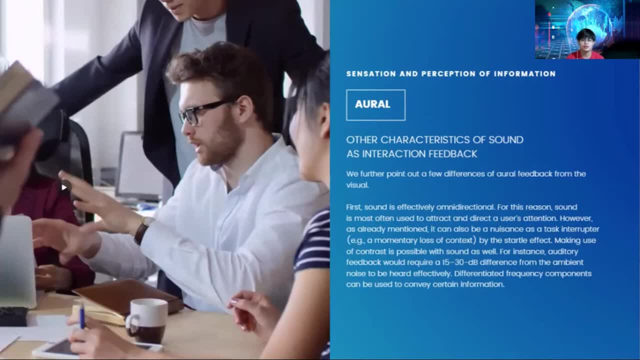 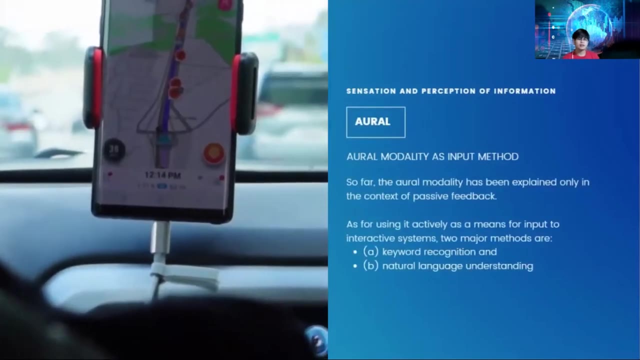 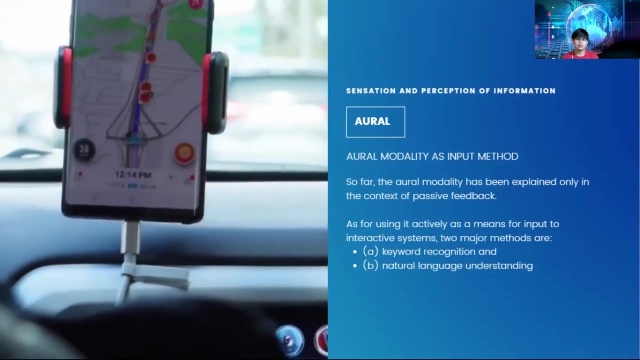 a 50 to 30 decibels difference from the ambient noise to be heard effectively. okay, so differentiated frequency components can be used to convey certain information. next, when it comes to oral modality as input method, so far the oral modality modality has been explained only in. 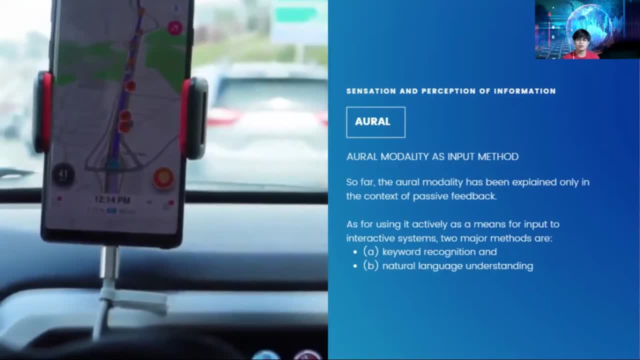 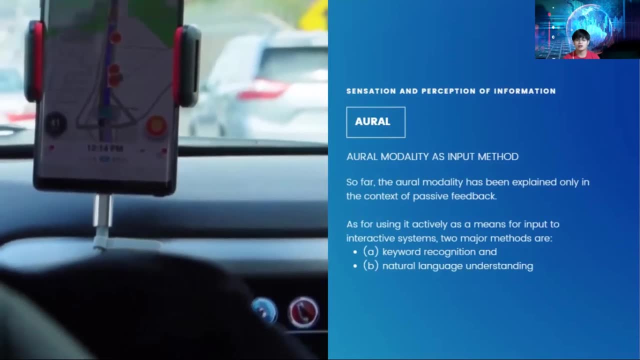 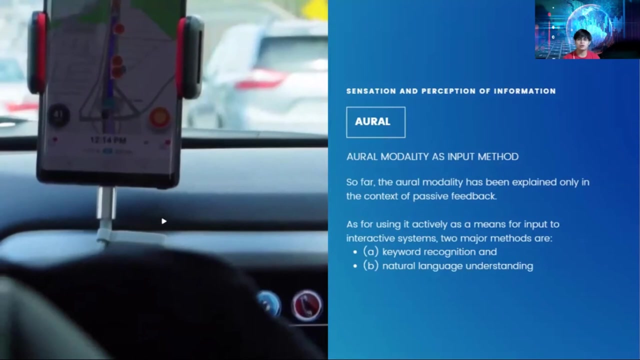 the context of acid feedback. so as we're using it actively as a man means to input to interactive system, so major methods are like a word recognition, natural language understanding, so I believe you're familiar with the voice commands most of your applications. no, okay. Google, okay, so it uses our sound, okay. and then yeah, keyword. 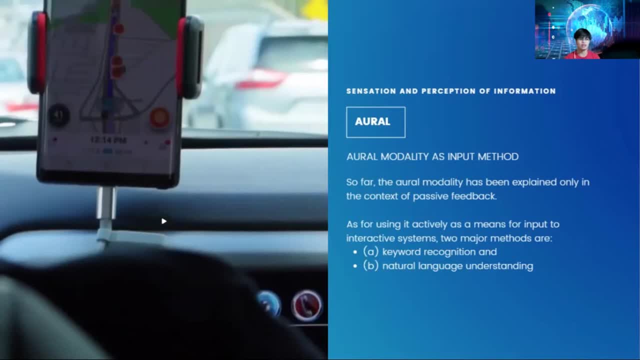 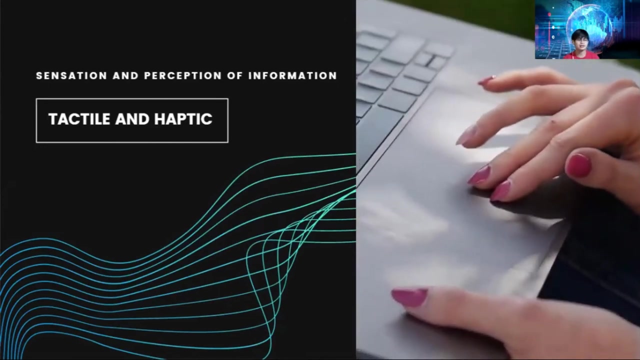 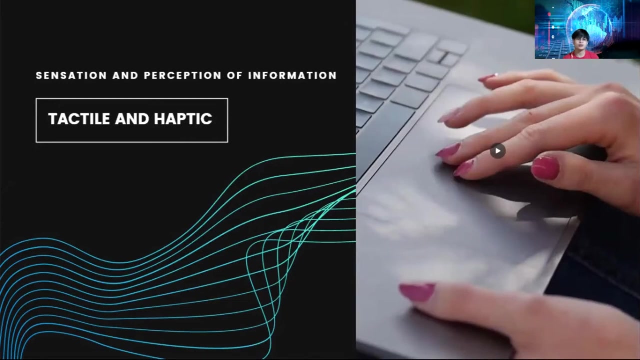 recognition. what would be different keywords in the linear action, not yet on my here. then the natural language understanding. okay, you need to, of course, understand, okay, so let's move on with the tactile and haptic. so when, actually, when we say tactile, haptic, it it's all about you know the sense of touch. so haptic is. 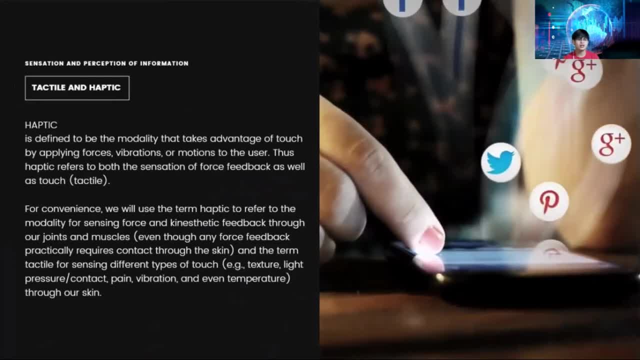 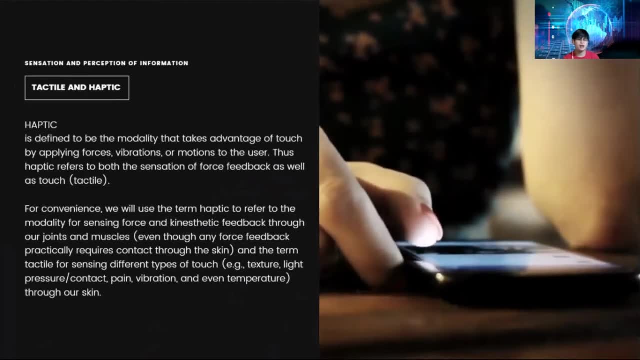 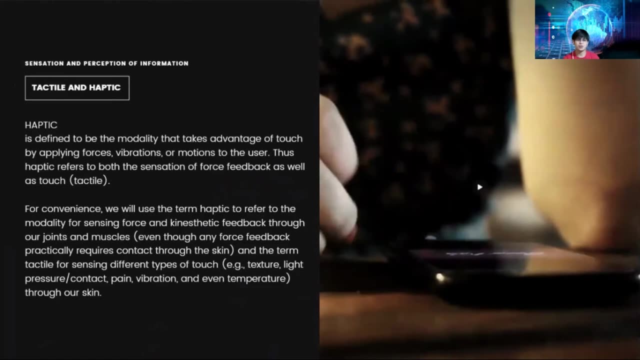 defined to be the modality that takes advantage of touch by applying forces, vibrations or motions to the user. thus, haptic refers to both the sensation of force feedback, as well as touch or tactile. so when you say tactile it is they, when, when you are applying, you know a touch with your, touching, your, your. 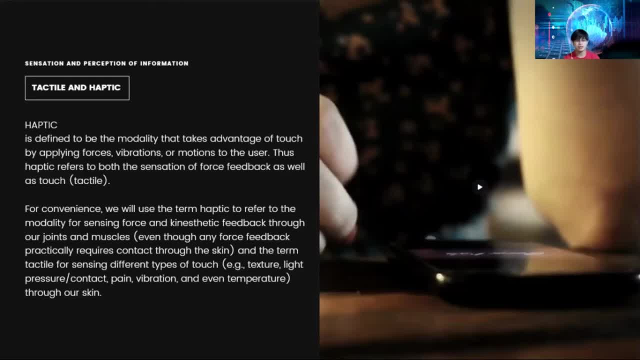 smartphone. okay, so when haptic, when, when, um, there's a sensation of force feedback with touch. okay, so, for convenience, we will use the term haptic to refer to the modality of sensing force and kinesthetic feedback through our joints and muscles, so even through any force feedback party. uh, practically requires contact. 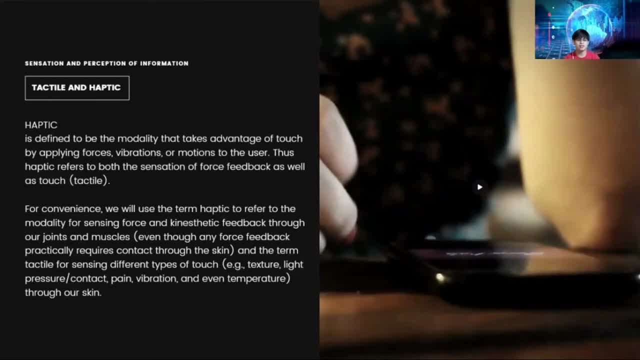 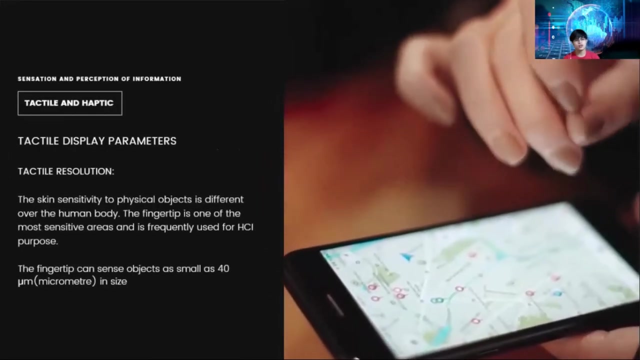 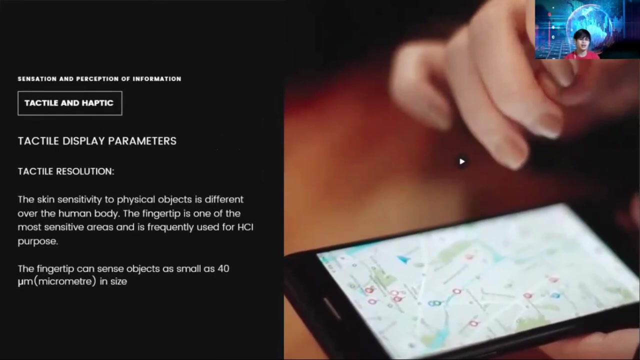 through the skin and the term tactile for sensing different types of touch- example texture, light, pressure, um contact, pain, vibration and event temperature- or through our skin. okay, so in a tactile. in a tactile there is the tactile display parameters, so the skin sensitivity to physical object is different from the human body. 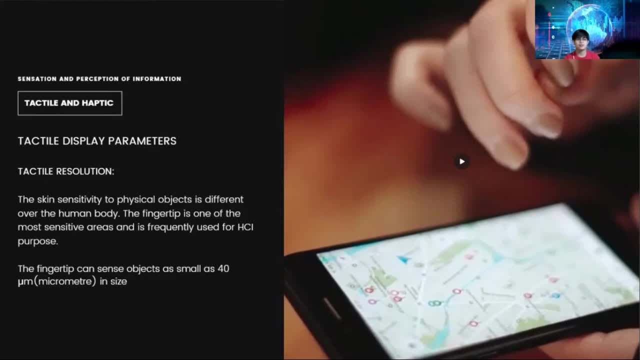 the fingertip is one of the most sensitive areas and is frequently used for HCI properties, so you may have observed negative touch screens to the fingertip. can can sense object, okay, and in my fingertips now when I'm gonna come down, can sense object as small as 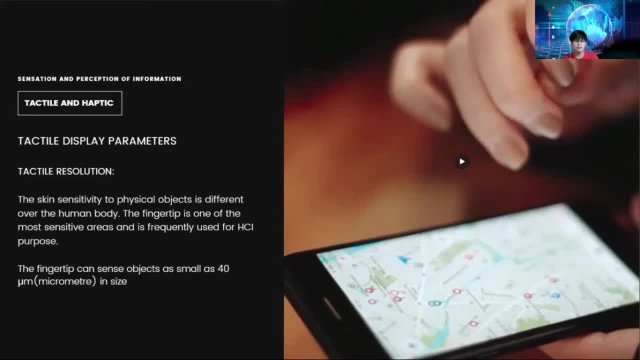 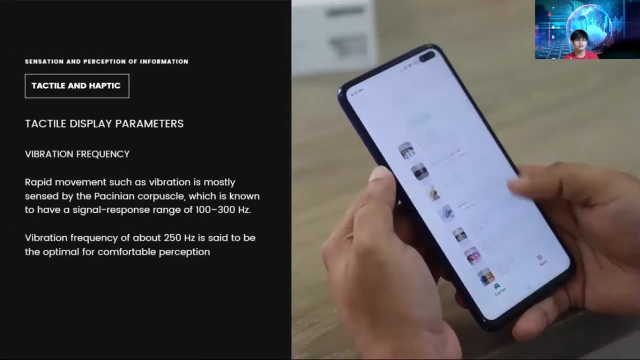 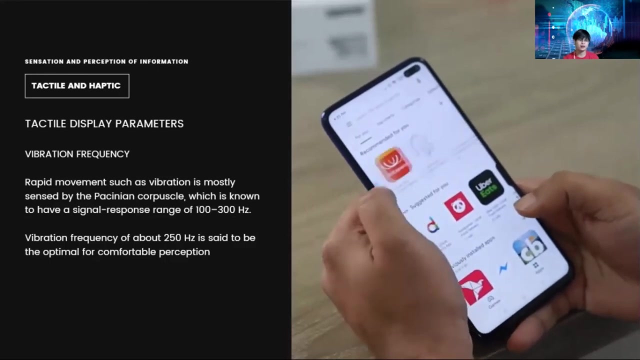 40 micrometer in size. so if you touch because I'm on fingertips would be um night interaction. okay, so the vibration frequency in a vibration frequency, rapid movements such as vibration, is mostly sensed by the Bosnian car Pascal, a bicycle, which is known to have a signal. 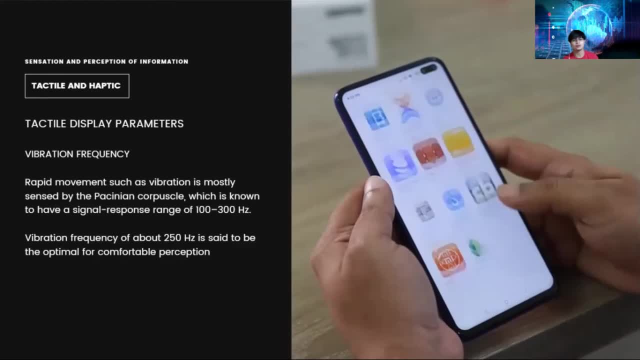 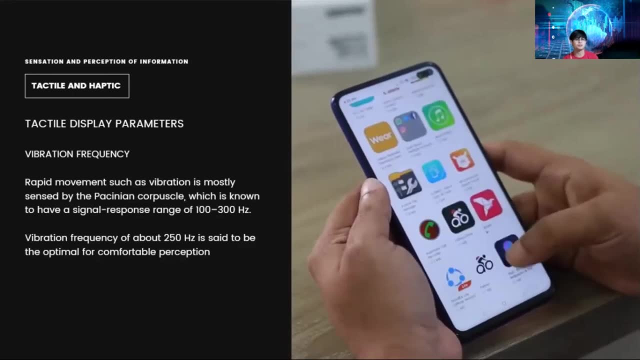 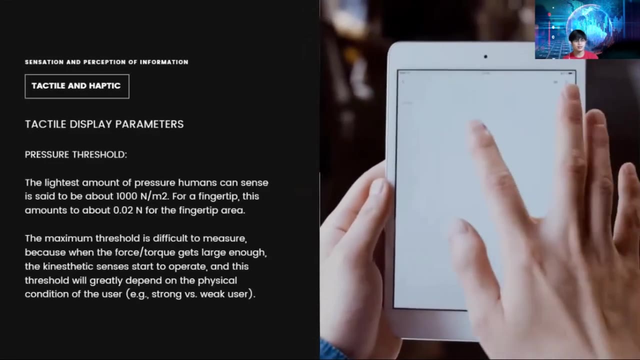 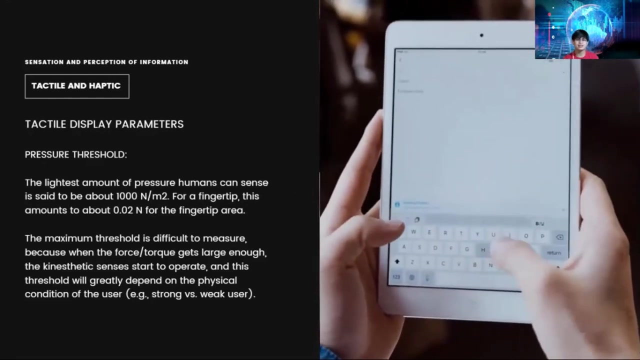 response range of 100 to 300 Hertz. so vibration frequency is about 250 Hertz is said to be optimal for comfortable perception. okay, so there is a vibration frequency. next is the pressure threshold. the pressure- the lightest amount of pressure humans can sense- is said to be about 102 squared. 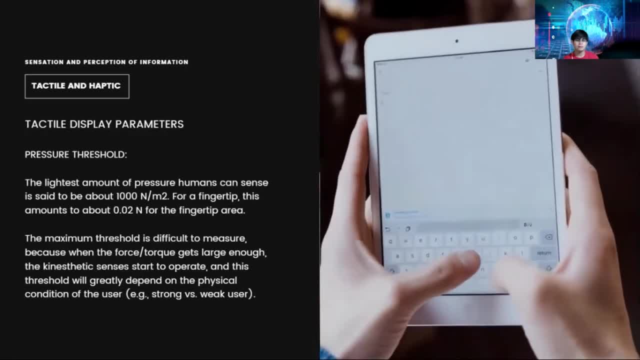 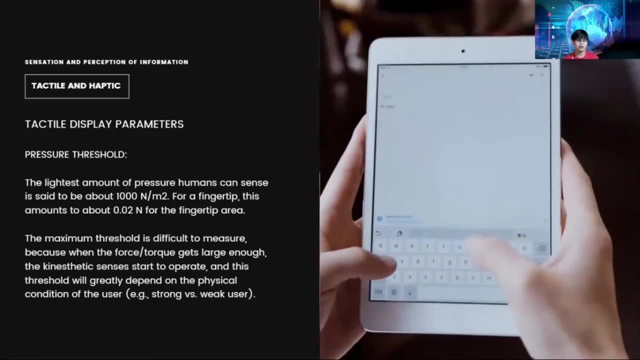 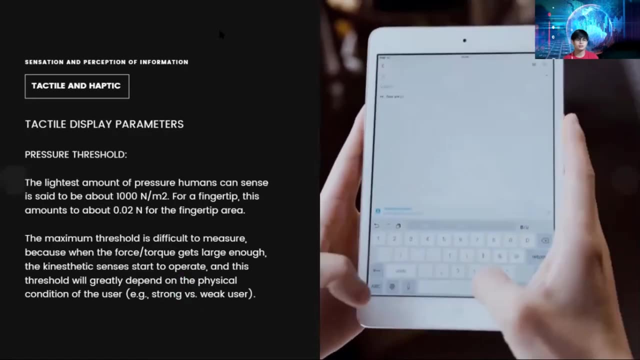 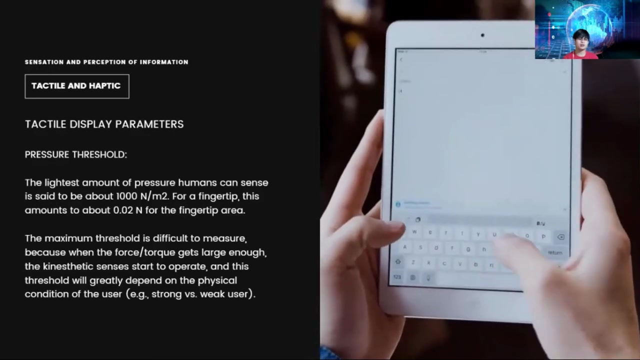 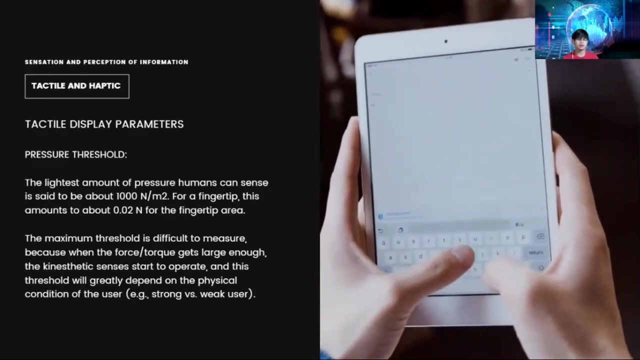 okay, so for a fingertip this amount is about 0.02 and for the fingertip radiant, okay. by the way, when we say n slash m, squared this, that Newton, or Newton per meter squared, that is the unit used in the touch. so the maximum threshold is: 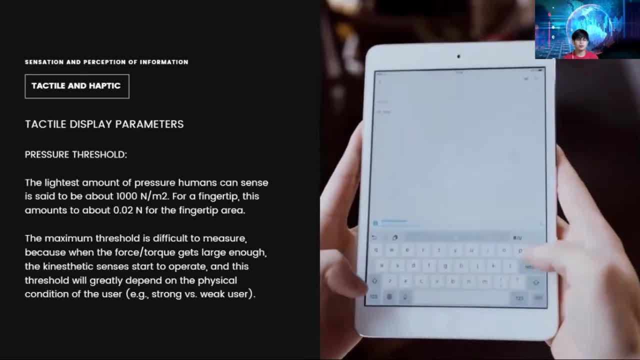 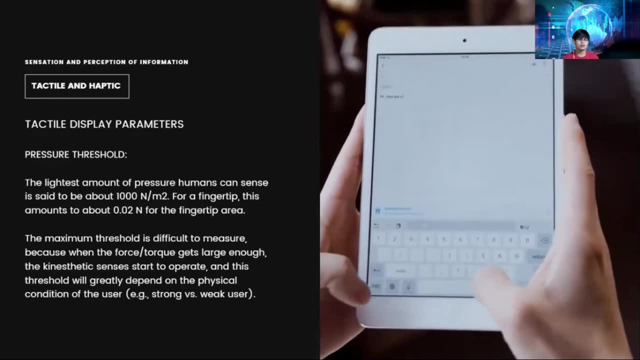 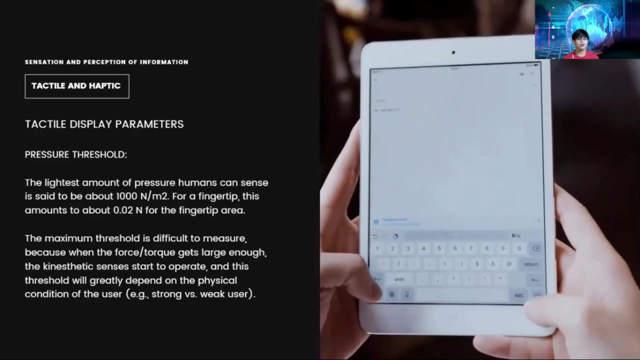 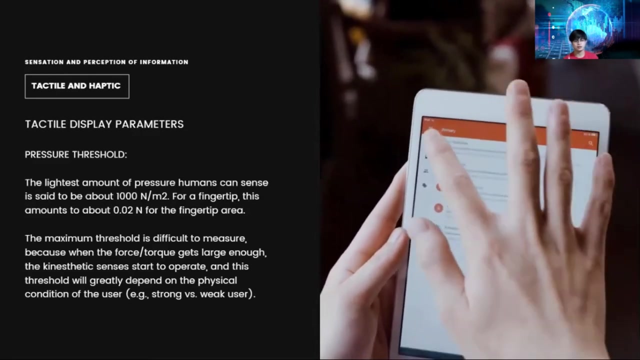 difficult to measure because when the force or torque gets larger enough, they can aesthetic sense are to start to operate. so, on, this threshold will greatly depend on the physical condition of the user, whether strong versus a weak user. okay, so again, just learn basic concept. when it comes to the pressure, 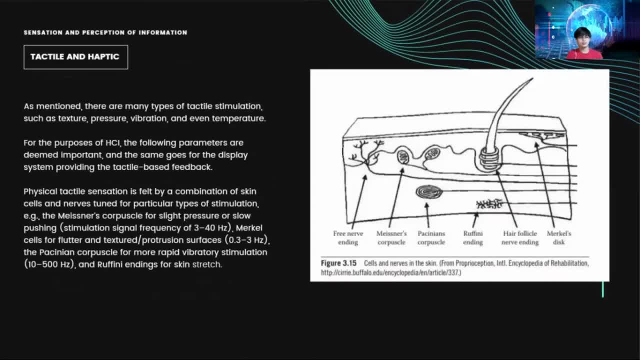 threshold. so, as mentioned, there are many types of a tactile stimulation, such as the textural pressure, pressure, vibration and even temperature. okay, so for the purpose, for the purposes of HCI, the following parameters are deemed important in the same goals for the display system providing the tactile based feedback. 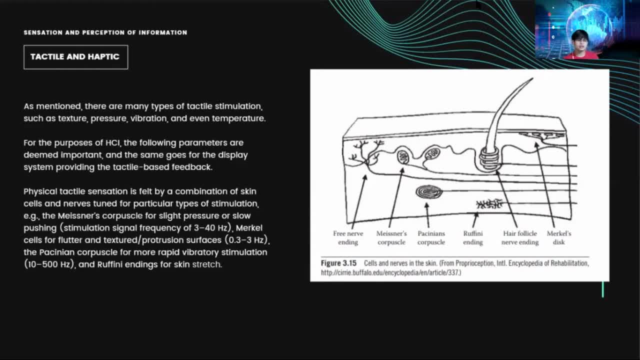 okay. so physical, tactile sensation is filled by a combination of skin cells and nerves tuned for a particular touch. types of stimulation example: the missionary corpus call for slide pressure or slow pushing, or this simulation signal: frequency of three to four Hertz. mercozoles to Flutter and textured. 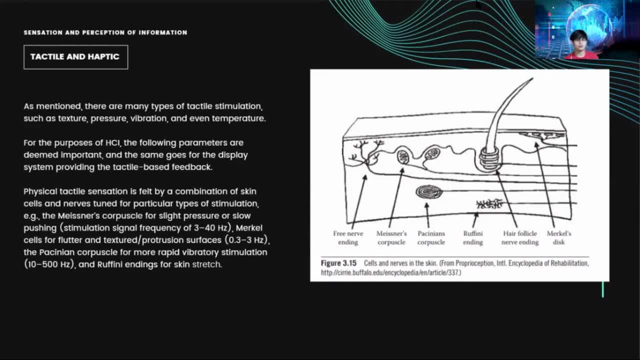 broad uh quadrillion services or 0.3 to 3 Hertz. the pacinian corpus call for more rapid laboratory simulation to from one or from 10 to 500 Hertz. androphenia endings for skin stretch. so medium and guys, you guys know, but um, just got to know the basic. you know more like, so, so some. 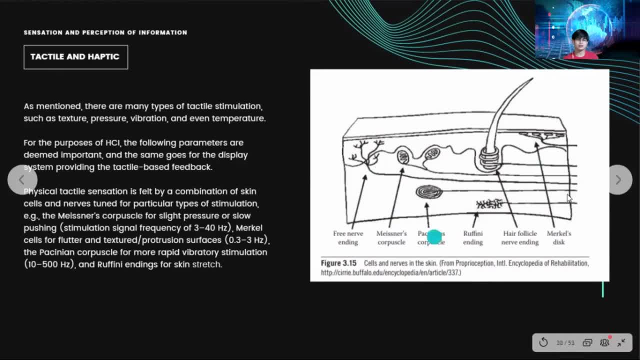 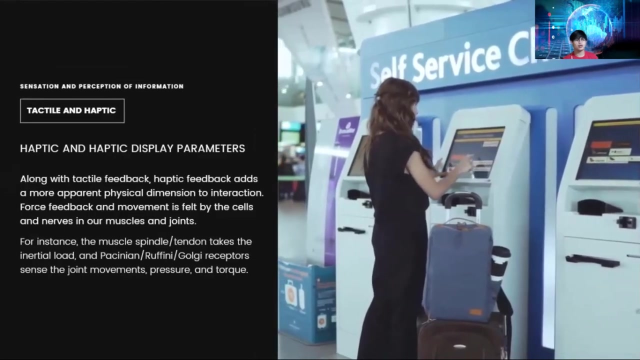 nerves in the skin. okay so, um, again, we will not, really didn't have enough of to deeply discuss. you know, if you want to learn more about skin, then search it in Google and study the different parts. okay, so let's move on with the next slide. okay, so along with the tactile. 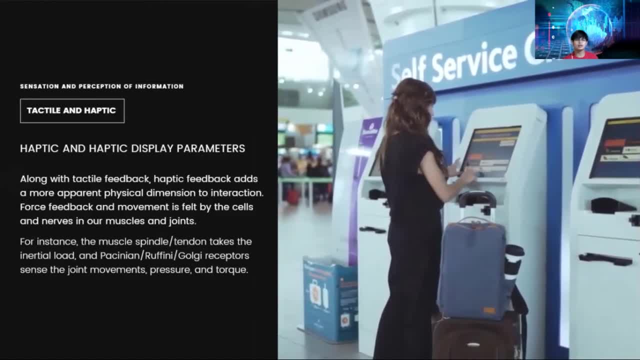 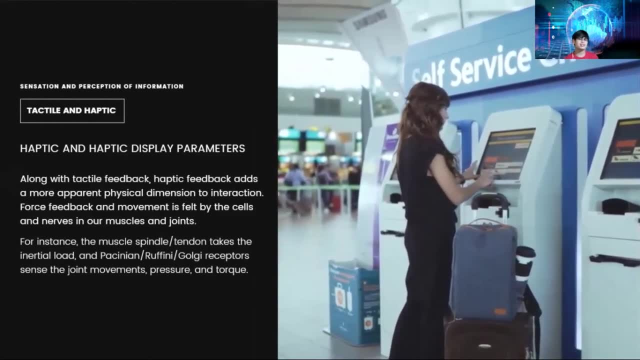 feedback. haptic feedback adds a more apparent physical dimension to interaction. so force feedback and movement is felt by the cells and nerves in our muscles and joints. for instance, the muscles, spindles or tendon takes the inertial load and the pacinian orrophenia or Golgi receptors. since the joint movements pressure and 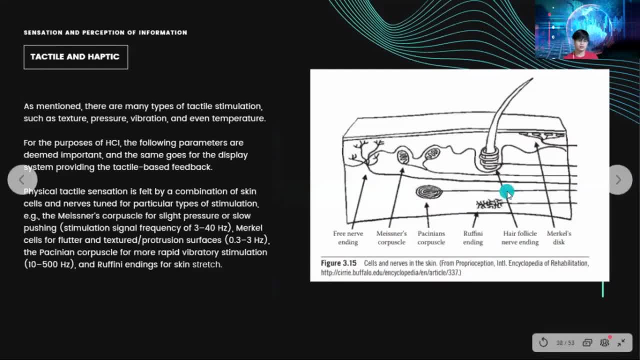 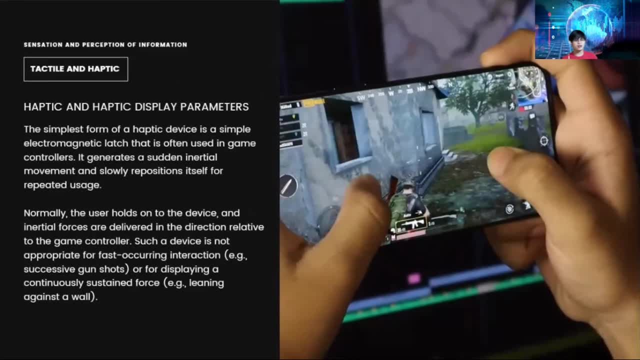 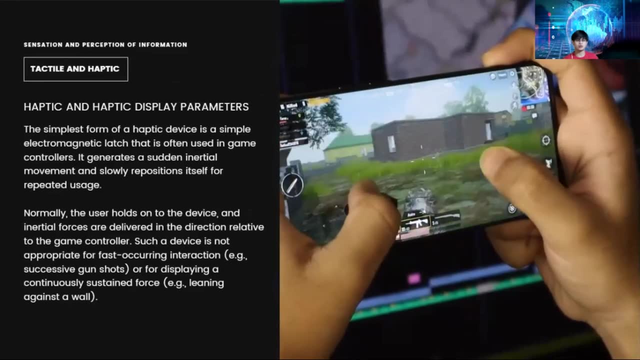 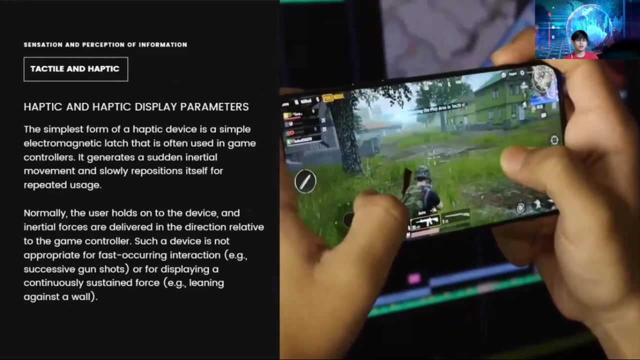 torque. so here it is okay. next, the simplest form of haptic device is as simple as electromagnetic latch that is been used in game controllers. so it generates a sudden inertial movement and slow reposition itself for a repeated user usage. normally the user holds onto the device and inertial forces. 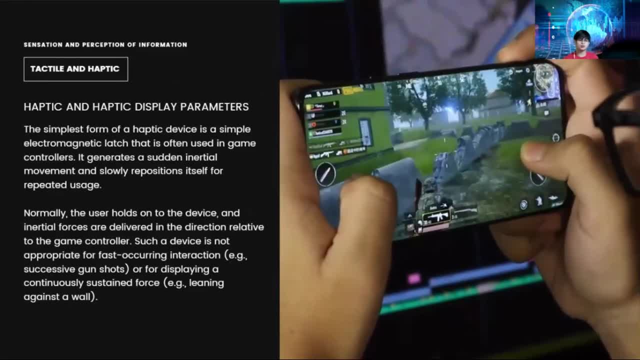 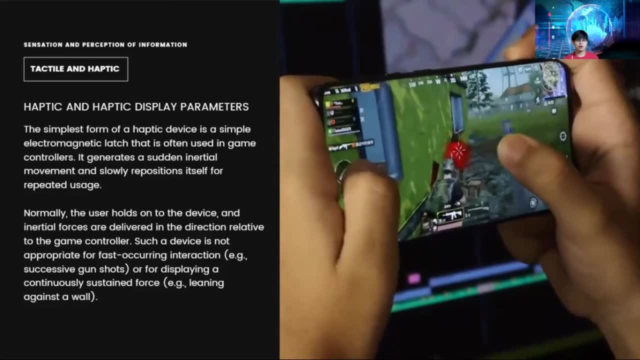 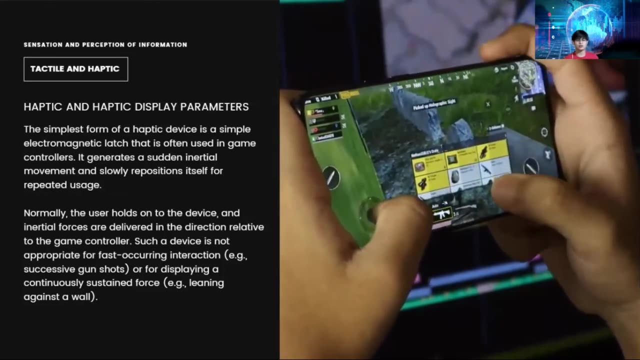 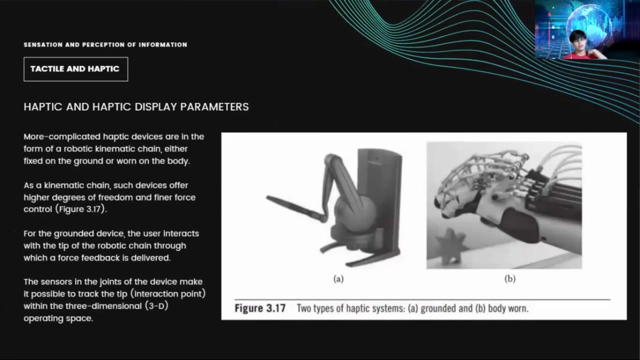 are delivered into direction related to the game controller. such a device is not appropriate for a fast acquiring interaction or, um example, successive gunshots, or for playing a continuously sustained force, for example just leaning against a wall. next, more complicated haptic devices are in the form of robotic kinematic chain, either fixed on. 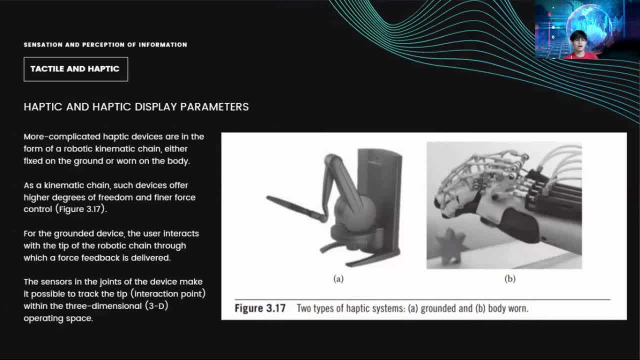 the ground or worn on the body, so as kinematic chain. such devices offer higher degrees of freedom and finer force control. you can see, this is our example, okay, figure 3.17. so for the grounded device, the user interacts with the tip of the robotic chain, through which, of course, feedback is delivered. so the sensors and 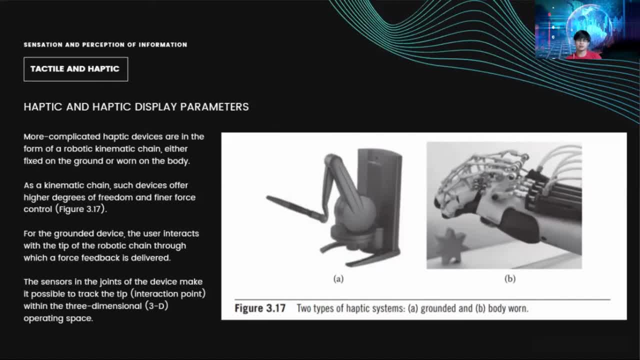 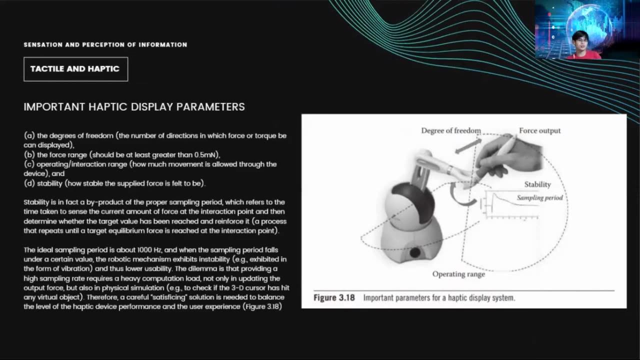 the joints of the device make it possible to track the tip or the interaction point within the three-dimensional rating space for 3D. so the important haptic display parameters are the following: the degrees of freedom, meaning this is the number of direction in which force or torque we can be displayed. 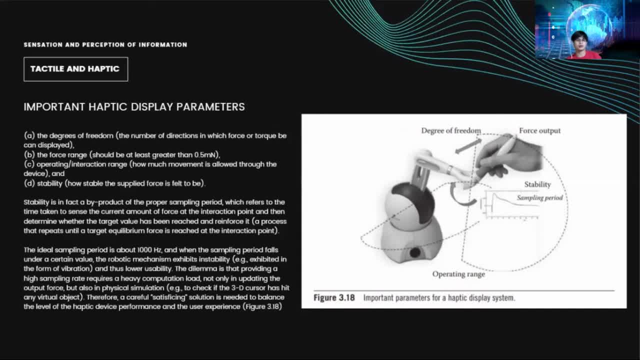 the force range, that is, should at least greater than zero point MN. the operating or interaction range, or how much movement is allowed through the device. and the stability. stability, or how stable the supplied force is, failed to be okay. the stability is, in fact, a byproduct of the 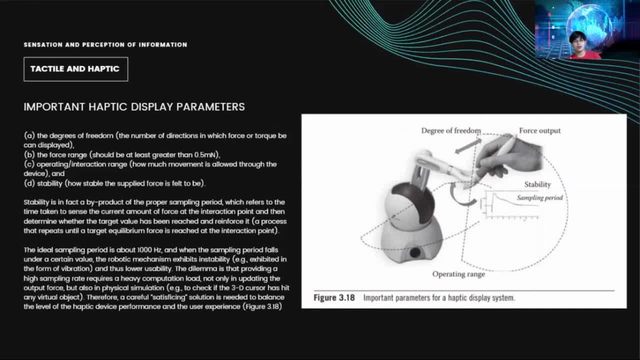 proper sampling period, which refers to the time taken to sense the current amount of force at the interaction point and then determine whether the target value has been reached and reinforced it. so it is a process that repeats until a target equilibrium force is reached at the interaction point. okay, so the ideal sampling period is about 1000 Hertz and 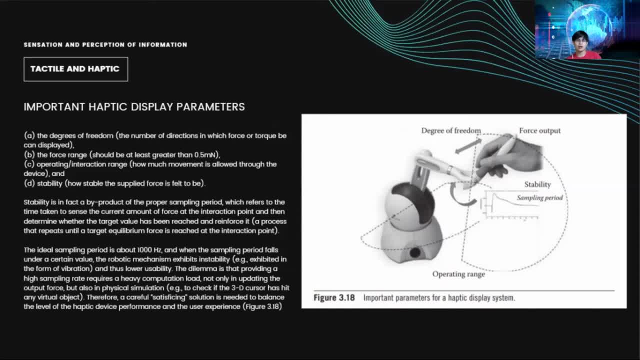 when the sampling period falls under a certain value, the robotic mechanism exhibits instability. okay, so, example: exhibited in the form of vibration and thus lower usability. so the dilemma is that providing a high sampling weight requires a heavy computation load, not only in updating the output force, but also physical stimulation. okay, for example, that we 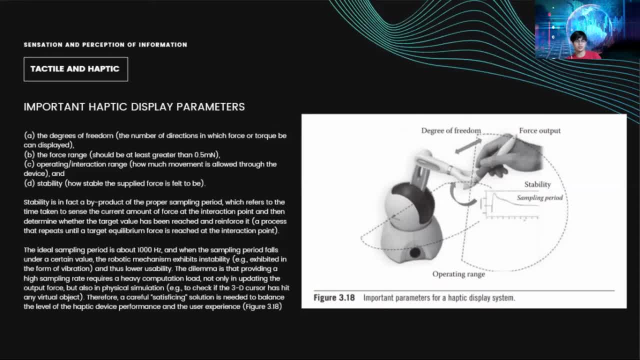 do check if the 3D cursor has set enabled full object. so therefore, a careful, satisfying solution is needed to be balanced: the level of the haptic device, performance and the user experience. so that's a sample illustration, for example, that this is the sample illustration for the camera and this is just a siblings or Aender app. and, lastly, to get a regular GPS managed with the haptic information. pour that in there, okay. so now, as usual, for protocol. evenly, a key factor, which obviously has many access and even modeling officially, is that code of labor which markets also four problems and often are sometimes poor and often we have吃h and occasionally even remove their 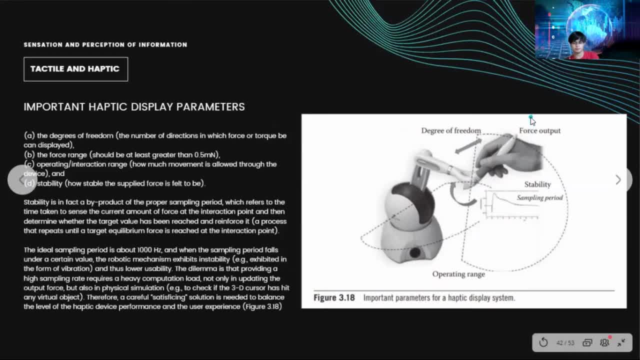 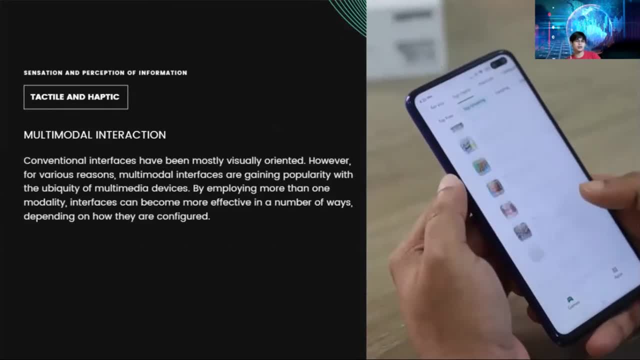 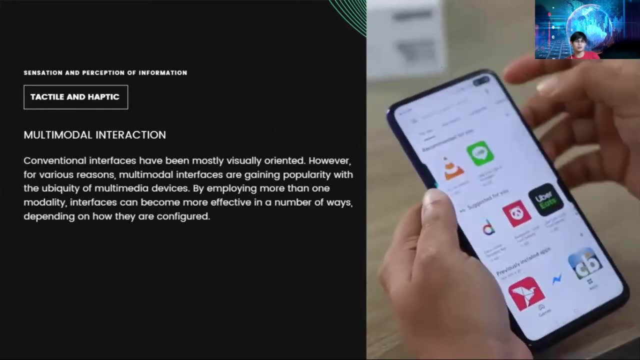 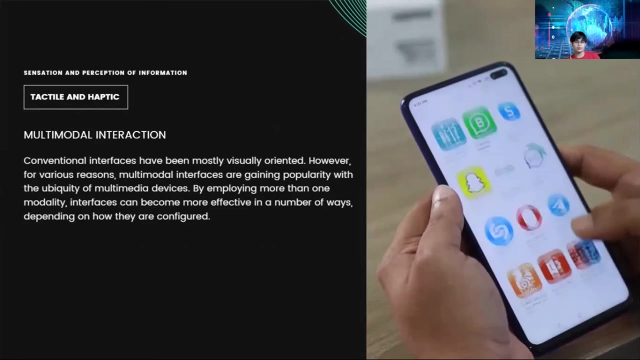 the sample illustration for that one. next, the multimodal interaction. so conventional interfaces have been mostly visually oriented. however, for various reasons, multimodal interfaces are gaining popularity with the ubiquity of multimedia devices. so by employing more than one modality, interfaces can be more effective in a number of ways, depending 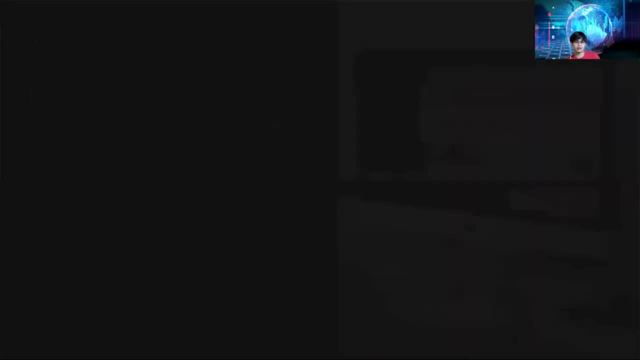 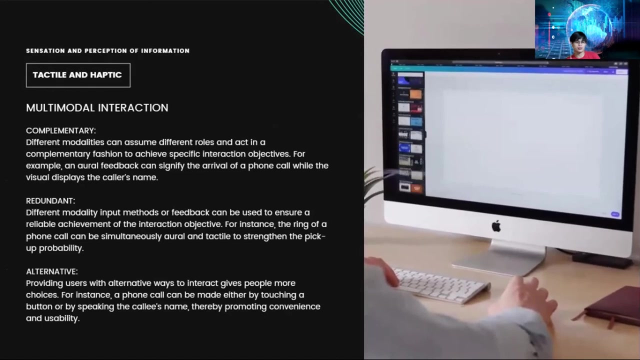 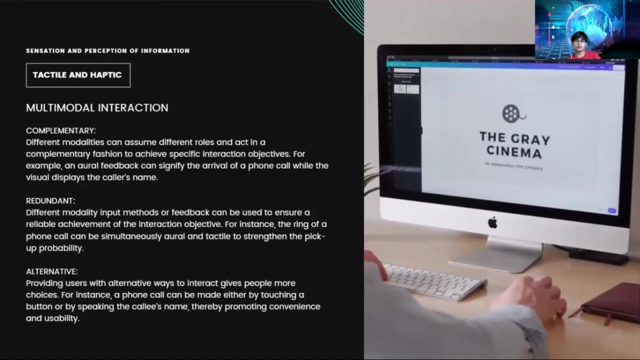 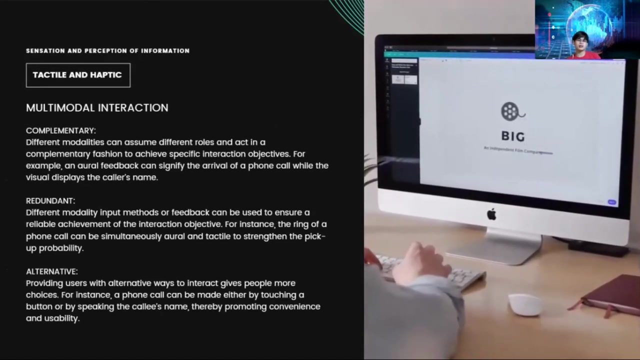 on how they are configured. okay, so in a multimodal interaction, there is its properties. first is the complementary. in the complementary, different modalities can assume different rules and act in a complementary fashion to achieve specific interaction objectives. okay, so, for example, an oral feedback can signify the arrival of a phone call, while the 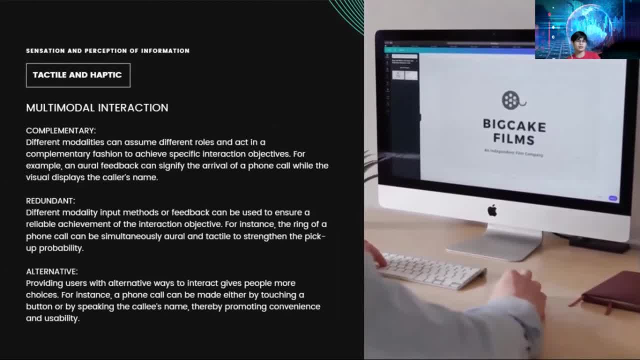 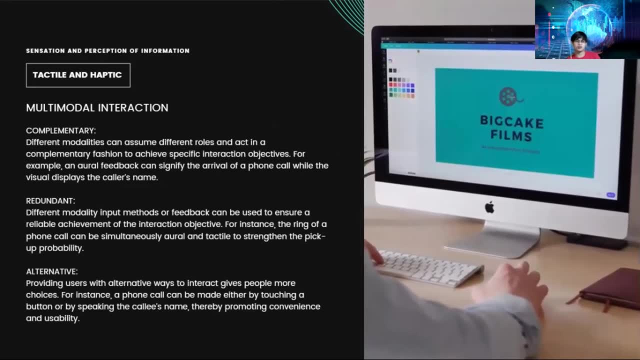 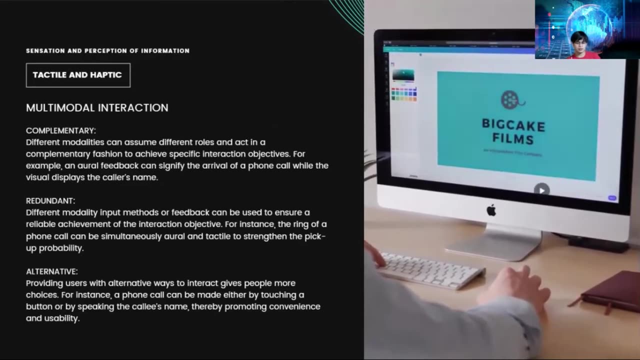 visual display the caller's name- okay, that is complementary- and then the redundant. redundant meaning different modality, input methods or feedback can be used to ensure a reliable achievement of the interaction object. so, for example, the ring of a phone call that can be simultaneously oral and tactile. to 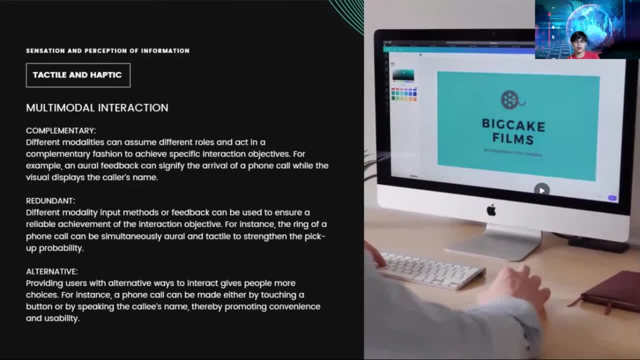 strengthen the pickup probability, okay, and the other one is the alternative. so using users with it with alternative ways to interrupt gives people more choices. so for instance, in the sample again, a phone call can be made either by touching a button or by speaking the caller's name, so thereby promoting 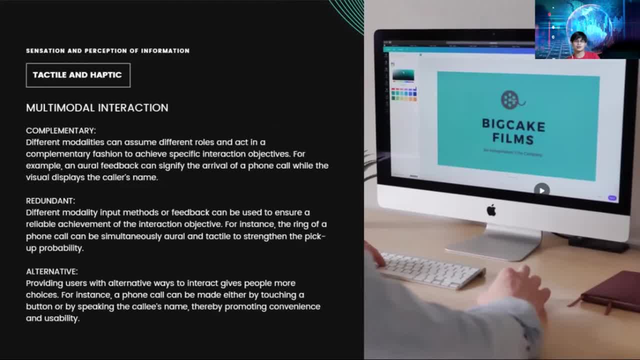 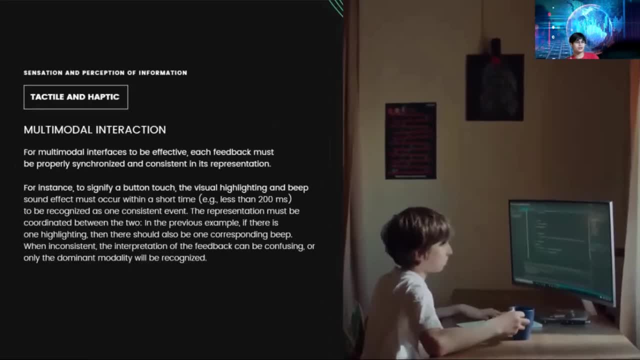 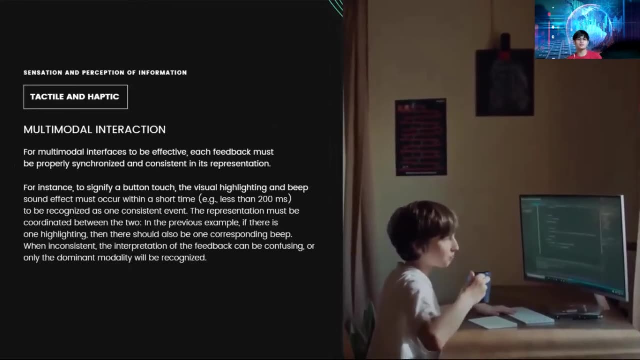 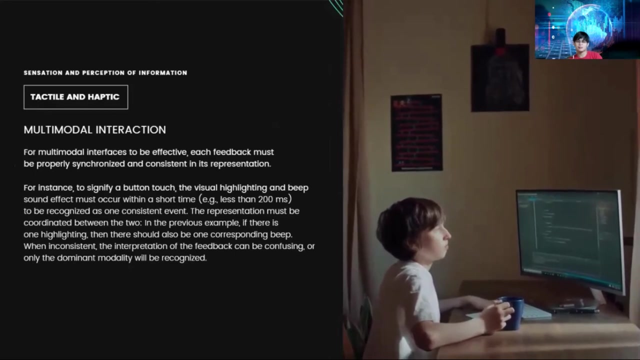 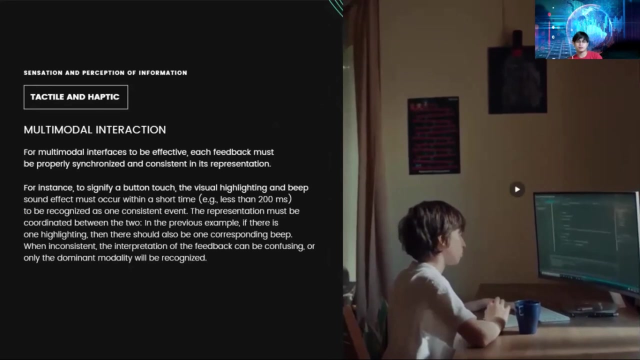 convenience and usability. so a multimodal interaction. okay, so for multimodal interfaces to be effective, each feedback must be properly synchronized and consistent in its presentation. so, for instance, to signify a button touch, the visual highlighting and beep sound must occur within a short period of time, so around less than 200 milliseconds be recognized. 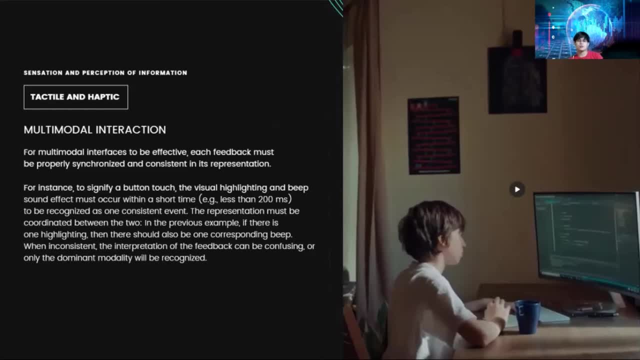 as one consistent event. okay, so the representation must be coordinated between the two in the previous example. if there is one highlighting, then there should also be a corresponding beep. okay, when inconsistent, the interpretation of the feedback can be confusing, for only the dominant modality would be recognized. 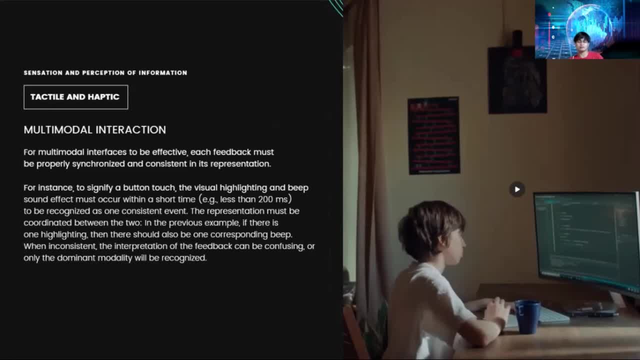 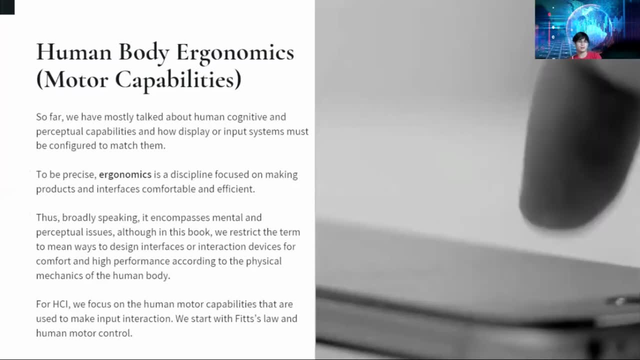 between you know the interface, and then the oral and gigamic, okay, the human body ergonomics or the motor capabilities. so we're gonna learn the basic principles, okay. so so far we have mostly talked about the human cognitive and perceptual capabilities and how display or input system that must be configured to match them. so, to be precise, 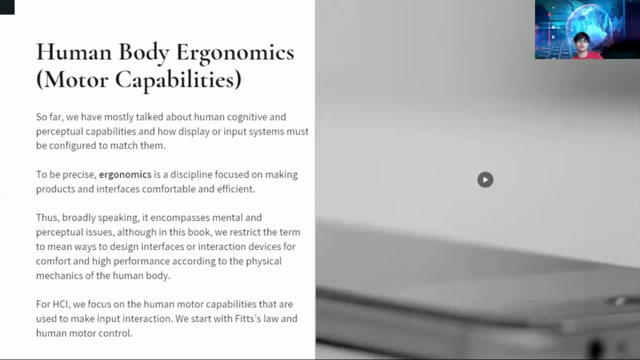 is a discipline focused on making products and interfaces comfortable and efficient. thus, broadly speaking, it encompasses mental and perceptual issues, although in this book we restrict the term to mean ways to design interfaces or interaction devices for comfort and high performance according to physical mechanics of the human body. for HCI, we focus on the human motor capabilities. 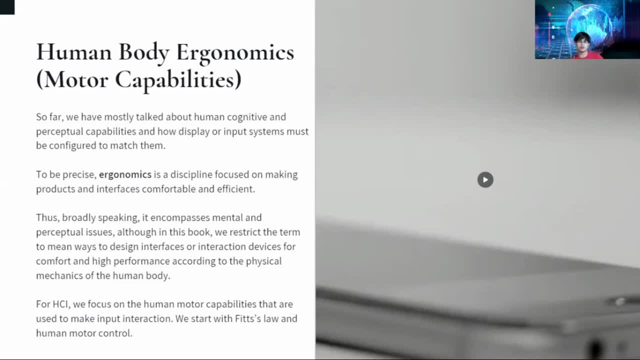 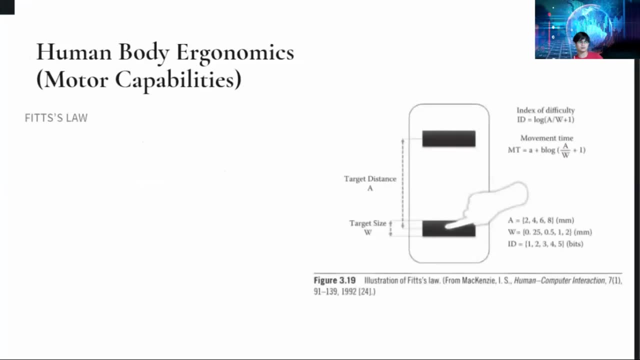 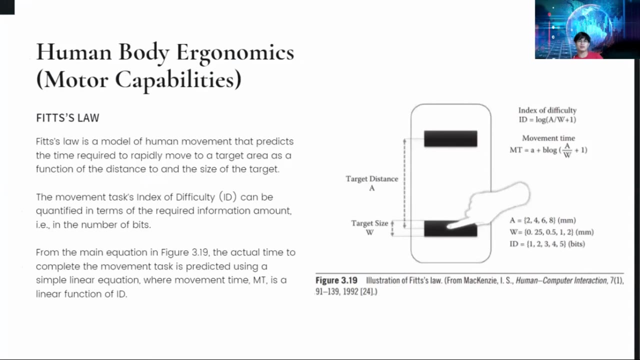 that are used to make input interactions. so we start with a FITS law and human motor control. okay, what is a FITS law? the FITS law is a model of human movement that predicts the time required to rapidly move to a target area as a function of the distance to and the size of the target. okay, so the movement task. 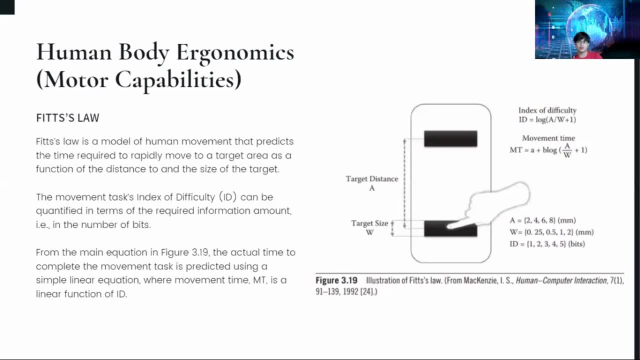 index of difficulty, or ID, be quantified in terms of required information amount in the number of bits. so from the main equation in 3.19, just look at the equation. the actual time to complete the movement task is predicted using a simple linear equation where movement time, mt, is a linear function of id. 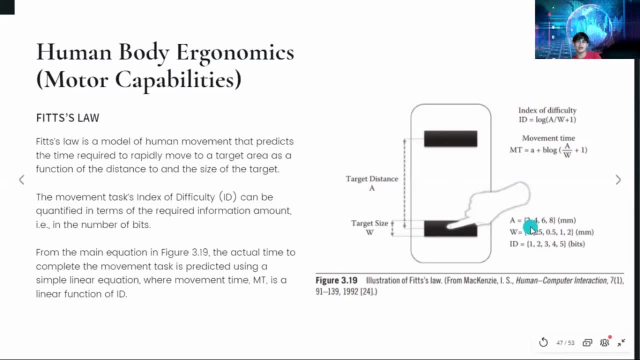 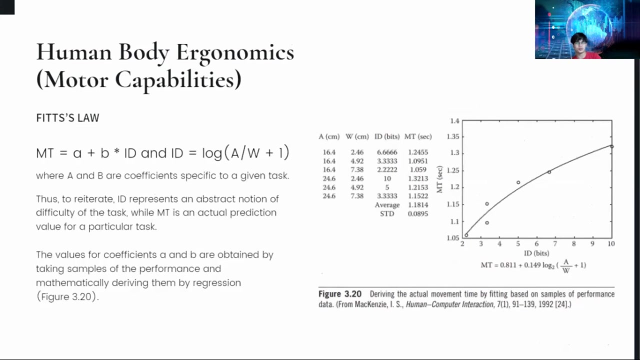 okay. so again, the predict the movement task is predicted using a simple linear equation where movement time, mt, is a linear function of id or index of difficulty. okay, so here's the formula. okay, mt is equal to a plus b multiplied by id, and id equals to the love joe. this is you know. so don't worry guys, there will be no calculation. 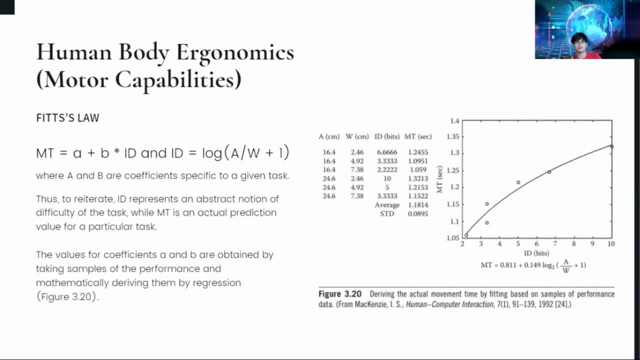 but it's gonna get the, the basic principle of the fit slow, okay. so, um, this is a formula where a and b are coefficients specific to given task. thus, to reiterate it, index of difficulty represents an abstract notion of difficulty of the task, while mt is an actual prediction value of 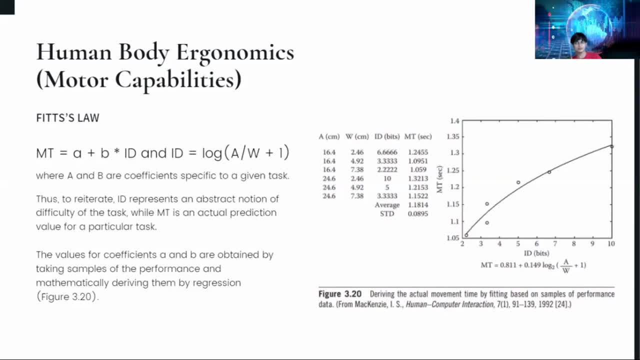 a particular task. okay, so the values for coefficients a and b are obtained by taking samples of the performance and mathematically deriving them by regression. this is the sample illustration. this is illustration, guys, um, deriving the actual moment time by fitting based on samples, performance data. okay, so again, no in in in hci. 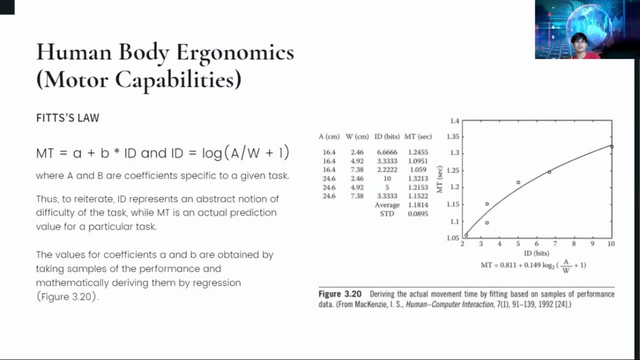 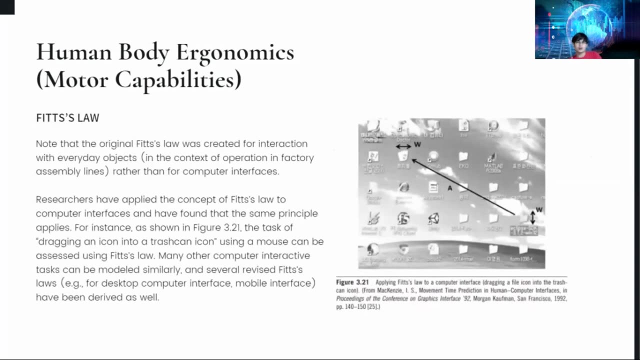 uh, principles, okay, note that the original switch law was created for interaction with everyday objects- okay, in the context of operation and factory assembly lines, rather than for computer interfaces. so researchers have applied the concept of fitch o to computer interfaces and have found that the same principle. 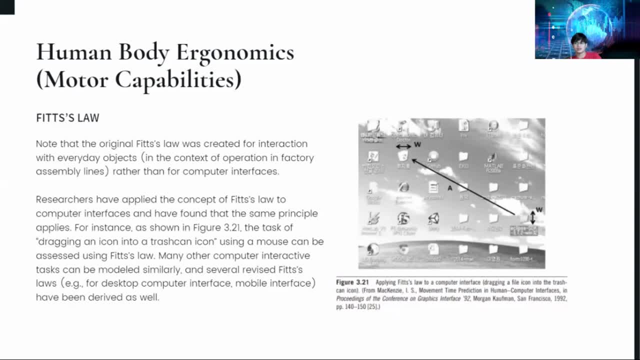 applies. so for instance, you know in a sample in in the figure that you're seeing, the task of dragging an icon into a trust scan icon using a mouse can be assessed using fits low. okay. many other computer interactive tasks can be modeled similarly in several revised fix law examples for desktop computer interface. mobile interfaces have been. 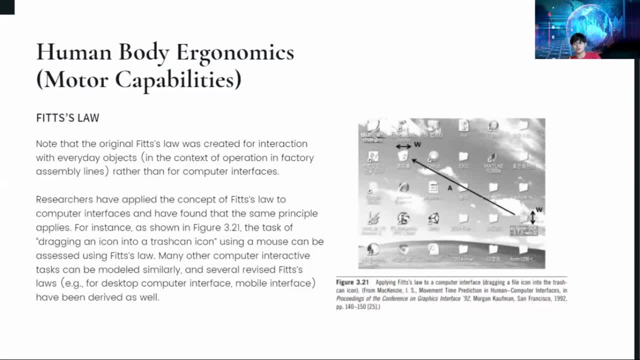 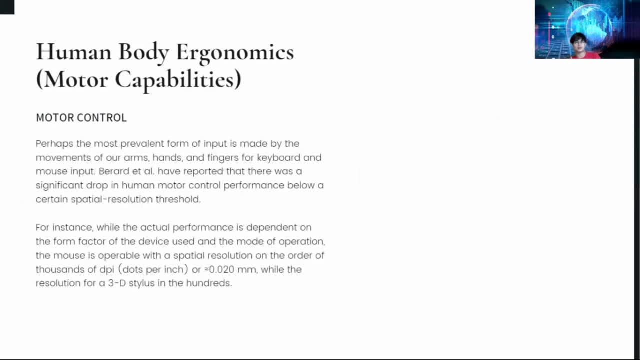 derived as well. okay, so we can meet and say that's a principal. next, let's discuss the motor control. perhaps the most prevalent form of input is made by the movements of our arms, hands and fingers now, or keyboards and mouse input, and even in the smartphones, depends upon what we werdenit require. iam molly know what your prepared for replacing. 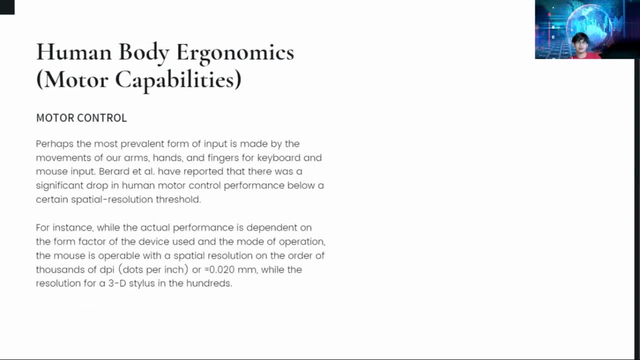 請 stan molly, Roma, Go for it. So Berard et al have reported that there was a significant drop in human motor control performance below a certain spatial resolution threshold. So, for instance, while the actual performance is dependent on the form factor of the device, 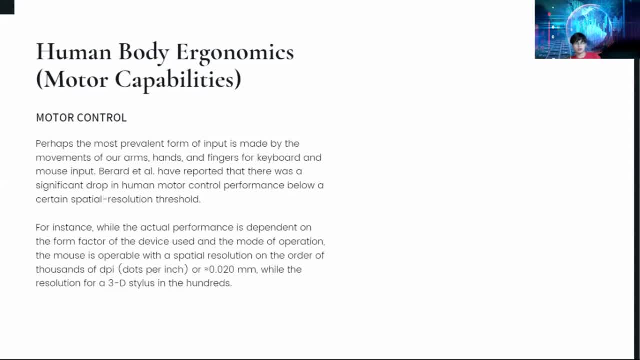 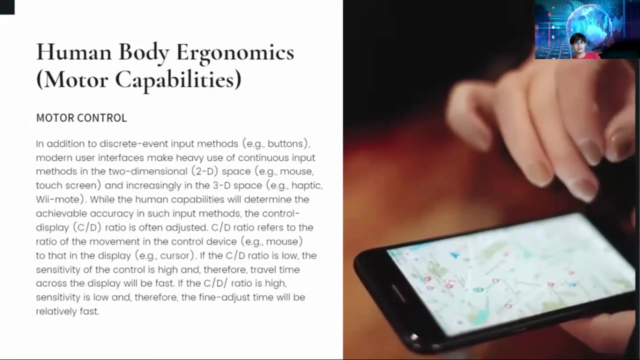 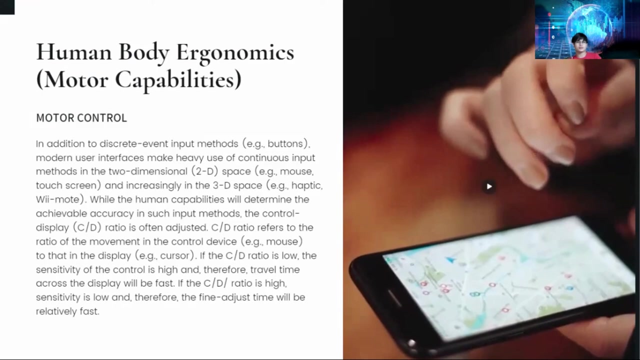 used in the model of operation the mouse is comparable with spatial resolution on the under of thousands of dpi, or that's per inch for 0.20 mm, while the resolution for a 3D stylus is in the handrails. Next, in addition to discrete input methods, modern user interfaces make 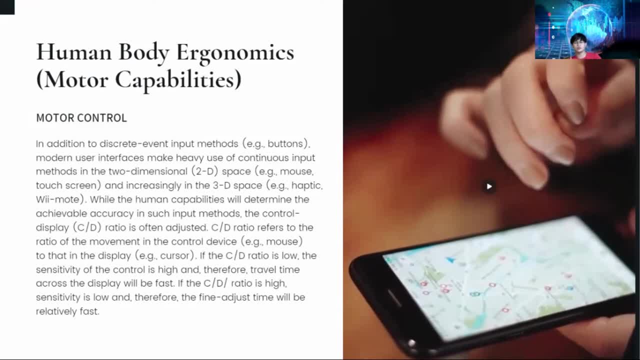 heavy use of continuous input methods in two-dimensional models, For example mouse touchscreen, and increasingly in the 3D space. while the human capabilities will determine the achievable accuracy in such input methods, the control display or CD ratio is often adjusted. 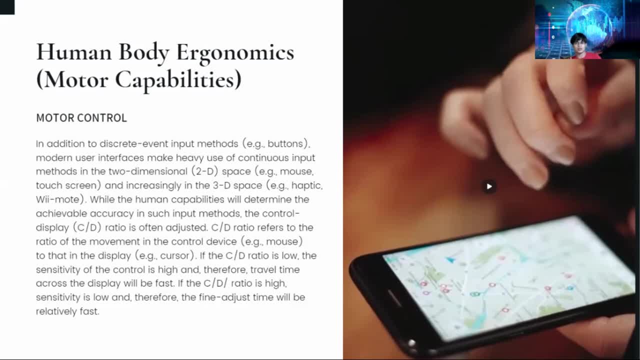 The CD or control display refers to the ratio of the movement in the control device to that in the display or cursor. If the CD ratio is low, the sensitivity of the control is high and therefore travel time across the display will be fast. 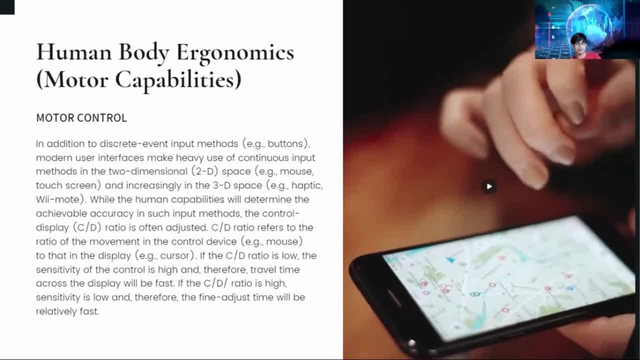 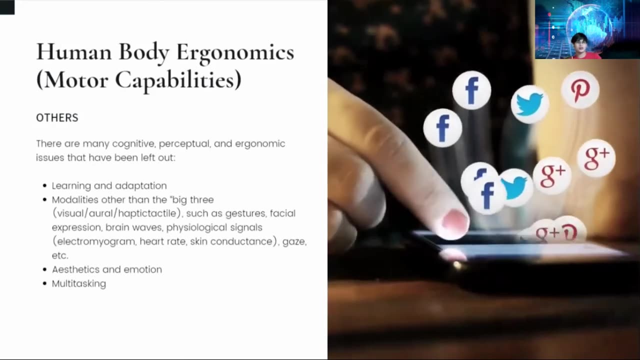 If the CD ratio is high, sensitivity is low and therefore the fine adjustment of the control device will be slow. just time will be relatively fast, okay, so as easy as that. and then the others. so there are many cognitive, perceptual and ergonomics issues that have been left out. learning and 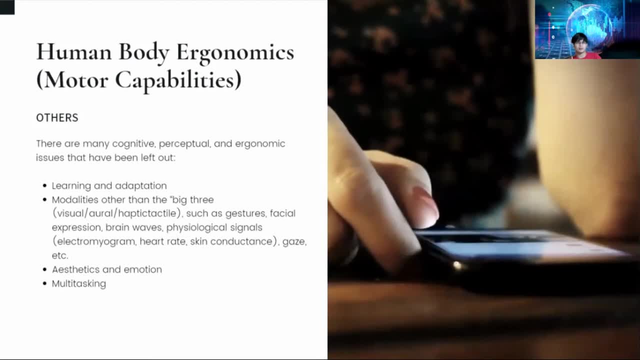 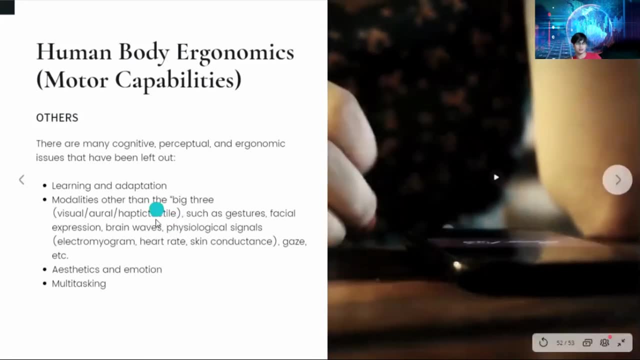 adaptation modalities other than the big three. we have visual, oral and haptic, haptic tactile. there's a space, actually must be here so- such as gestures, facial expression, brainwaves, physiological signals- and no I mean theological signals- and electromyogram heart rate scan, conductance gaze. 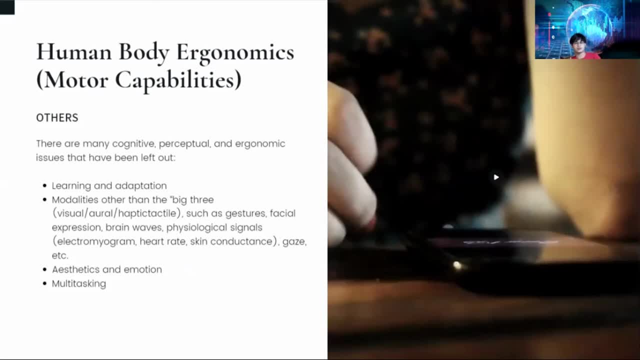 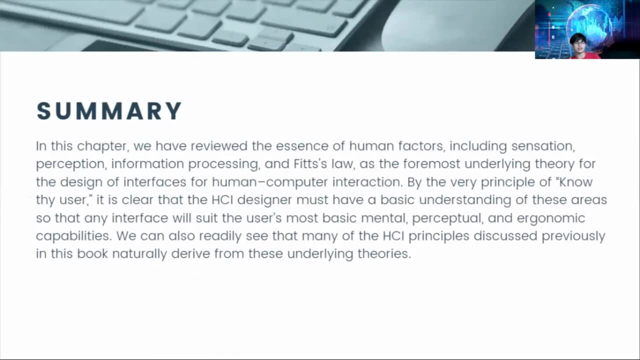 etc. and then aesthetics and emotion and multitasking. oh, oh. so that would be all for this chapter, okay, so in this chapter we have reviewed again guys, um, there might be things you know this would guys have done. just get the small concept. no, that when you actually design morning principle and the gamut, 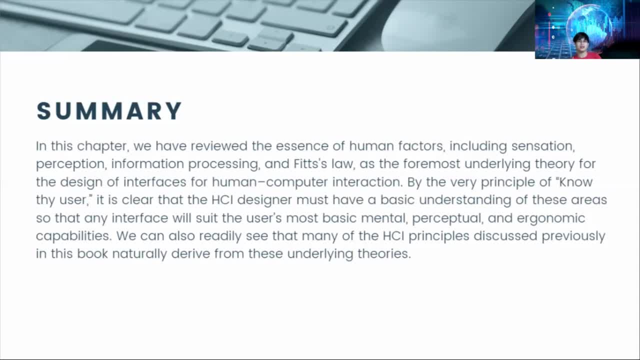 we use the. you know the, the eyes, the nose smell the ears. I think install, i mean the realue 예쁘 got your. So by the very principle of no-die user, it is clear that the HCI designer must have a basic understanding of these areas so that any interface will suit the user's most basic mental, perceptual and ergonomic capabilities. 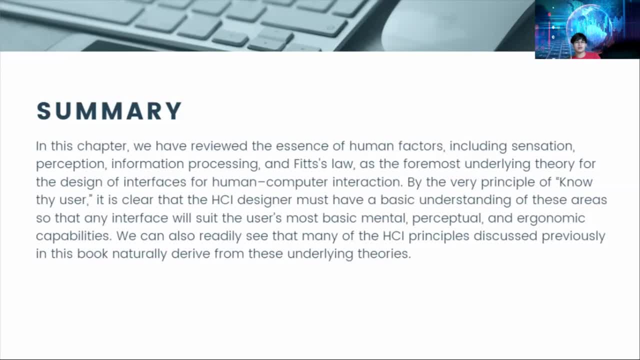 Okay, so we can also readily see that many of HCI principles discussed previously in this book naturally derived from these underlying theories. Okay, so I hope you guys have learned something. If there are things that at least you have done, then feel free to search more about that thing.